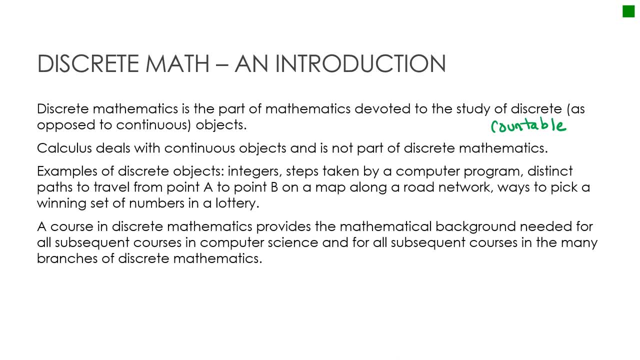 So I can list them, I can count them, etc. as opposed to continuous objects like we dealt with in calculus. So examples of discrete objects are integers, steps taken by a computer program, which is quite often why discrete mathematics is taken by those who are going into computer-based fields. 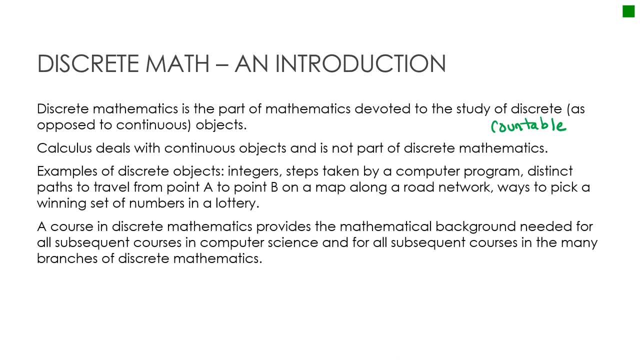 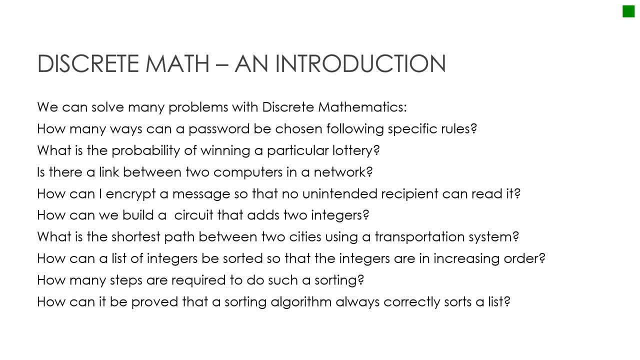 It basically is your foundation for the rest of the classes that you are going to need throughout your study at Bellevue University. On this slide I just wanted to give you the basics of the kinds of problems that we might solve with discrete mathematics. So some of these we will look at this term together and some we will not. 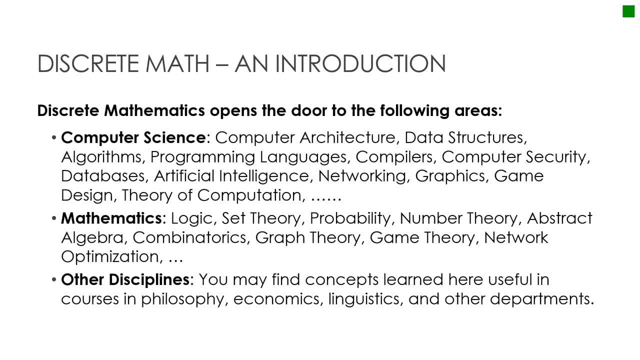 And essentially it opens the door to a lot of different areas. obviously, the study of mathematics, all of the things that we're going to learn- logic, set theory, probability, those of you moving on to combinatorics, which is my favorite class of all time- all of this is dealing with discrete math. 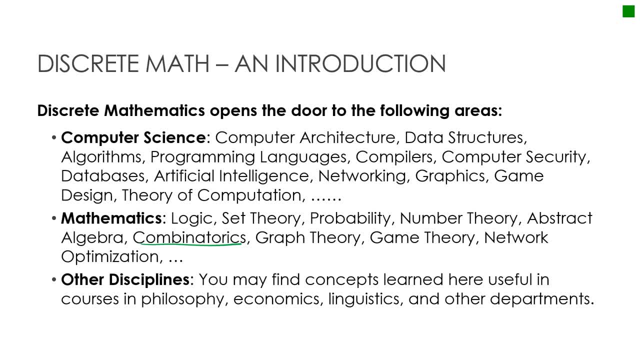 For those of you going the computer route. obviously it's a foundation for computer architecture, data structures, programming, etc. etc. and you can even find some of the applications that we're going to be talking about in this section. There are some applications of discrete in other areas of study as well. 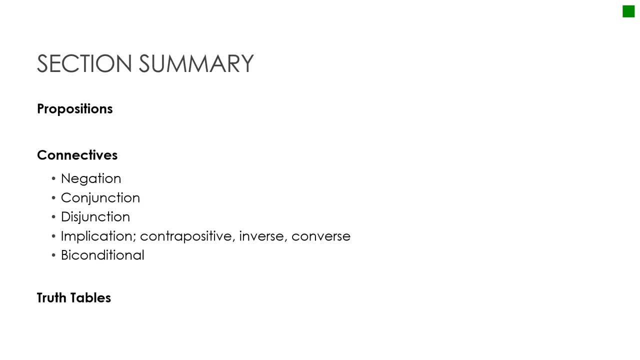 So section 1.1, propositional logic. In each section I provide a summary for you. Essentially, I do that so that it's easier for you, as the student, to go back to your notes and find exactly what we covered in each of these videos. 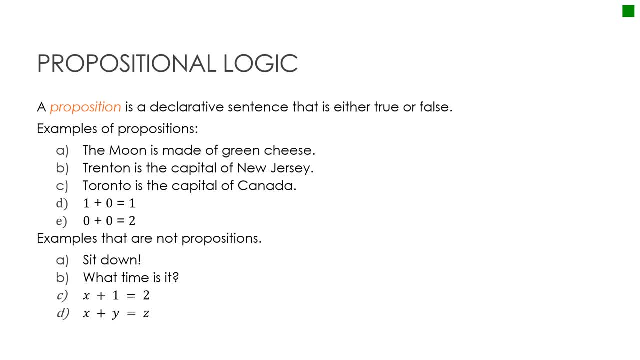 So a proposition is a declarative sentence. that is either true or false. The mood is made of green cheese. Obviously this is a false statement. Trenton is the capital of New Jersey. Toronto is the capital of Canada. 1 plus 0 equals 1.. 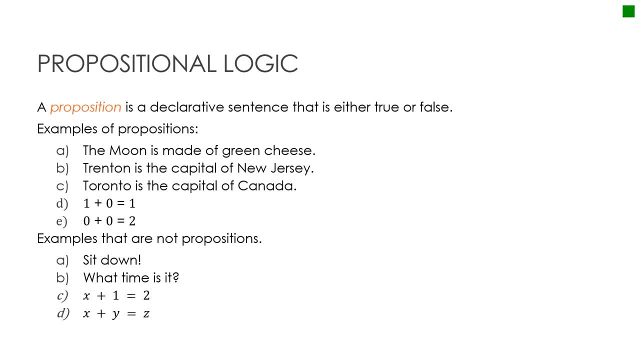 0 plus 0 equals 2.. Again, some of these are true, some are false. I'll let you determine which ones are which. Examples that are not propositions include, for instance, sit down, or what time is it, or the two equations that I have written for you. 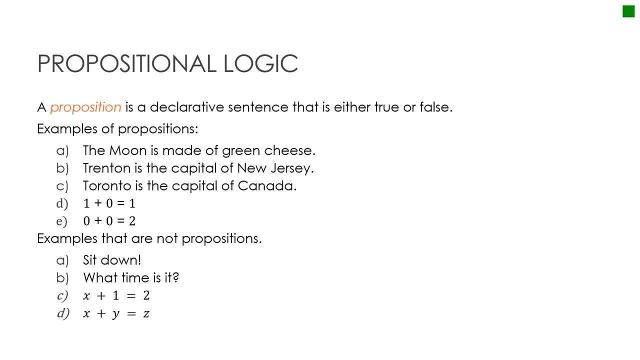 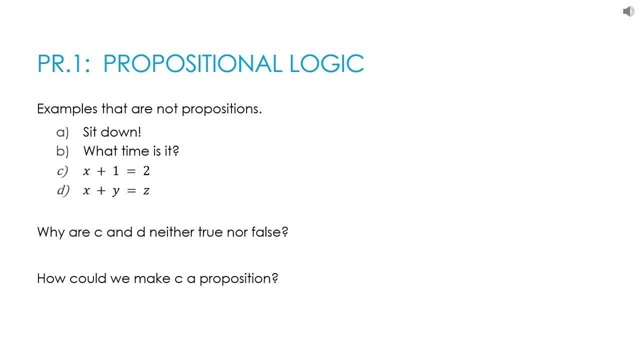 Now I want to talk to you a little bit more about those equations, but before we do that, I want you to have a chance to think about why. Okay, They are not propositions. Whenever we come to a slide where the title is written in blue and that's PR one or two, meaning practice one or two- in front of it, 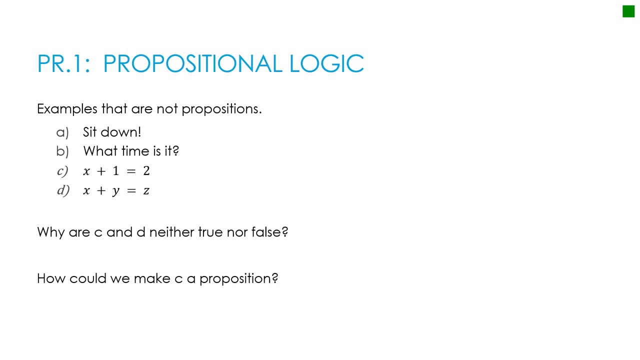 This is where I would really like for you to try the question on your own before I give you the answer. It's really important for students to actually try to think through these things before the answers are just given to them, because it doesn't require any struggle on your part and you won't actually learn anything. 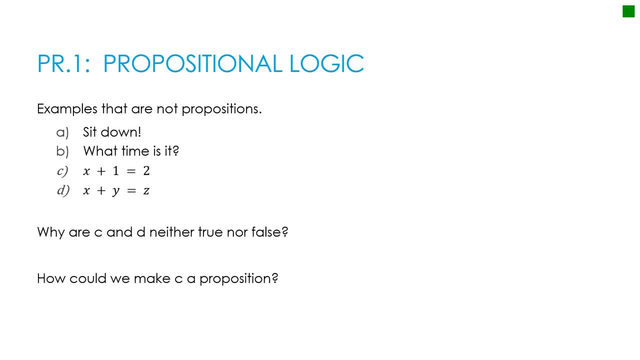 So whenever you get to one of these blue questions, Blue slides, I ask that you press pause, try the question and then, once you've either completed the question or you're just as far as you are able to get, then you press play to see how you did. 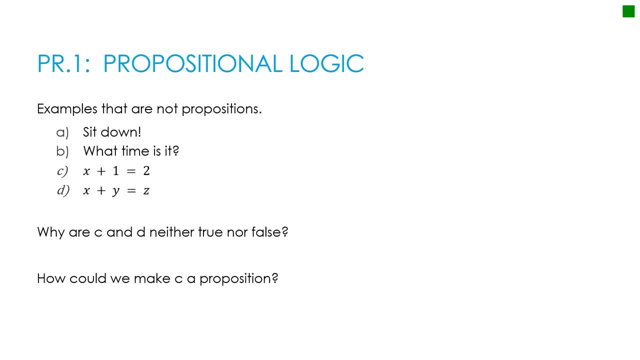 So if you haven't already, please press pause and we'll get started in just a minute. So hopefully you did press pause and you tried the question yourself. So I have two questions actually on this slide. The first is: why are C or D neither true nor false? 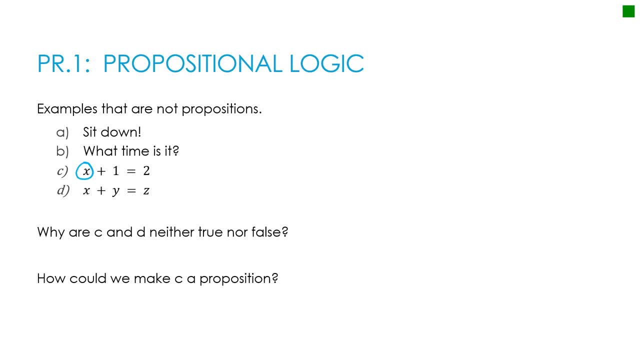 And in this case we're looking at our equations, And so in question C and in question D I have many variables. So in question C just one and in question D it's all variables. So why are they neither true nor false? It's because we have not yet assigned a value to the variable. 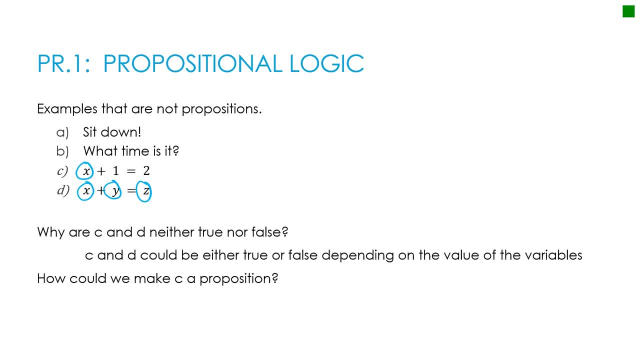 So why are they not? Because it could be true, depending on what value I put in. It could be false, depending on what value I put in. So how do we make C a proposition? Assign a value. So if I said x equals 3, now it's a proposition, even though it's a false one. 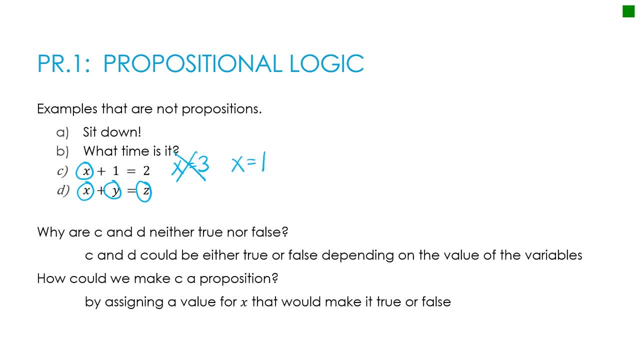 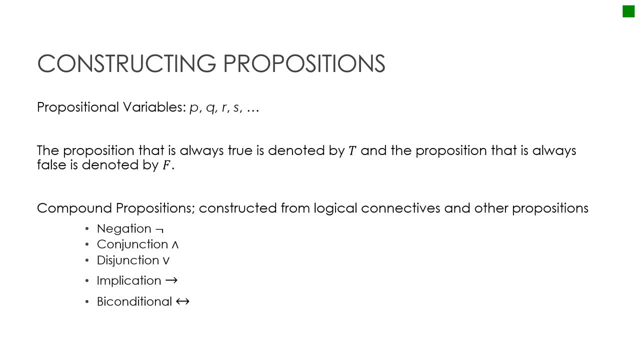 If I instead said: x equals 1, still a proposition. now it's a true proposition. So we're going to start constructing propositions And we have propositional variables And, just like in algebra, it doesn't really matter what you use, but most often you use x or y. 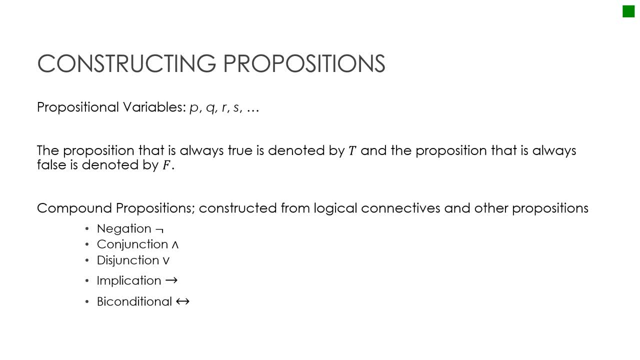 With propositional variables it doesn't matter what you use, But quite often we're using p, q, r, s, etc. Now the difference between a propositional variable and a variable that we use in algebra is: in algebra the variable represents a value or a set of values. 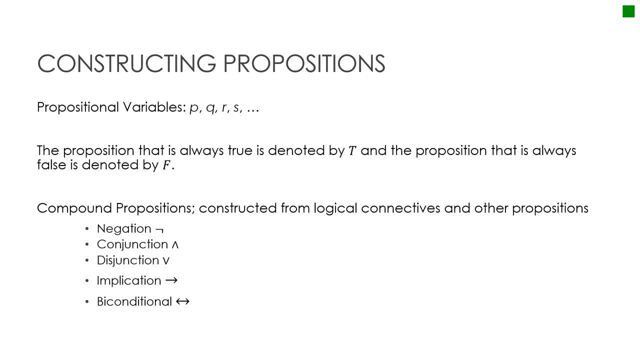 Whereas in discrete mathematics a propositional variable represents those statements that are either true or false. Now, if we have a statement that is always true, then it's okay for us to denote it with a t Always true. This proposition that's always false is obviously denoted with an f for false. 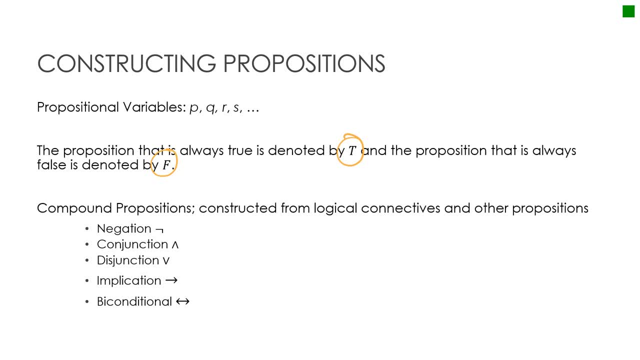 A lot of propositional statements might be true or false depending on the value or something else occurring in the problem, Just like when we looked at those equations a few moments ago. Now, compound propositions can really start to get confusing, So I would encourage you to spend some time just taking notes on these. 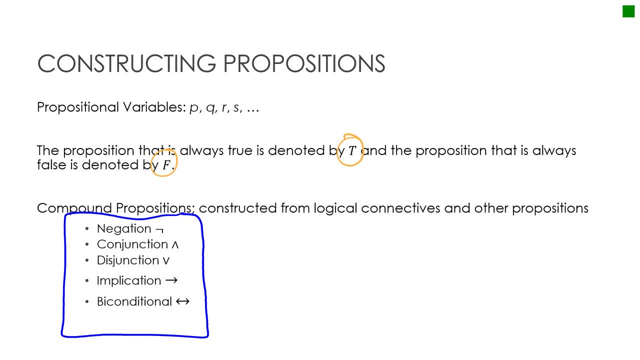 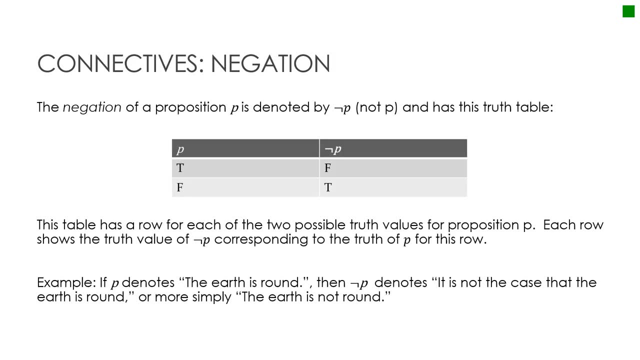 Or maybe making your own, Maybe making yourself a table to keep track of everything. But these are the compound propositions that we are going to be looking at in this course. So let's take a look at our first one, which is negation. The negation- usually I have that in orange, but negation of a proposition. 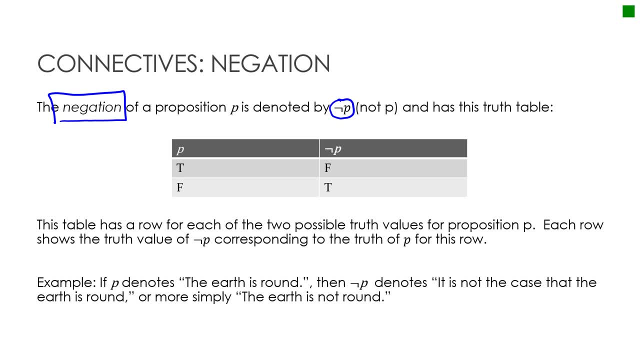 Note the notation that we'll be using. And we say that, not p, And then it says: oh hey, by the way, there's a truth table. Well, this is probably the first time you've seen a truth table, So let's talk a moment about it before we look at the values. 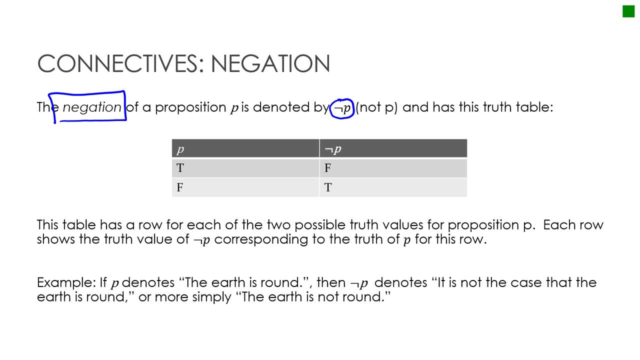 In a truth table, each row has all of the possible truth values for the proposition p. So obviously, with just one propositional statement, that statement is either true or false. So this is row one and this is row two. Each of them represents a different scenario. 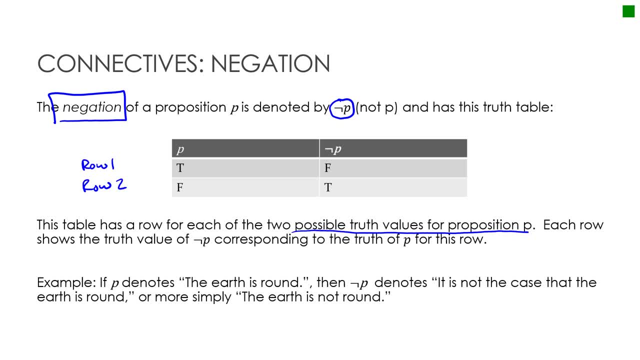 What the truth table says is: if p is true, then the truth value of not p is false. Whenever p is false, the truth value of not p is true. So we're looking row by row. So an example: if p- remember, p is a propositional statement. 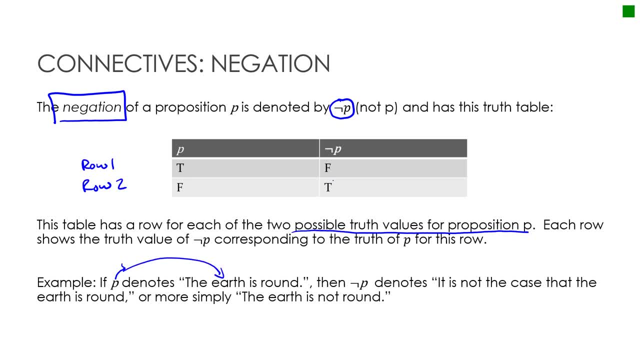 And say that statement is the earth is round. So that is a statement that is either true or false. Obviously it is true, Then not. p denotes that basically that it's not true. It is not the case that the earth is round. Or most of us write that a little bit more simply: the earth is not round. 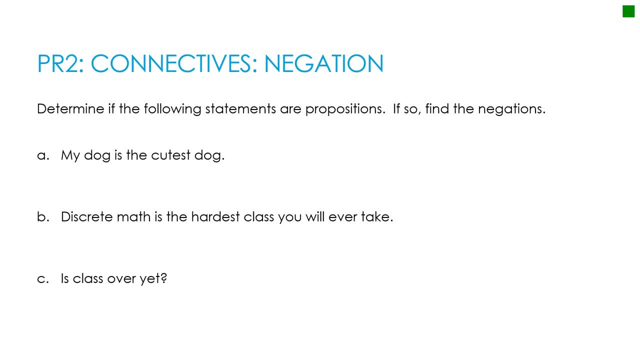 So again, here we arrive at a practice question, practice two, And the question is about connectives and negation. So my question is: are a, b and c are each of those propositions? if the answer is yes, it's a proposition, I would like you to find the negation. 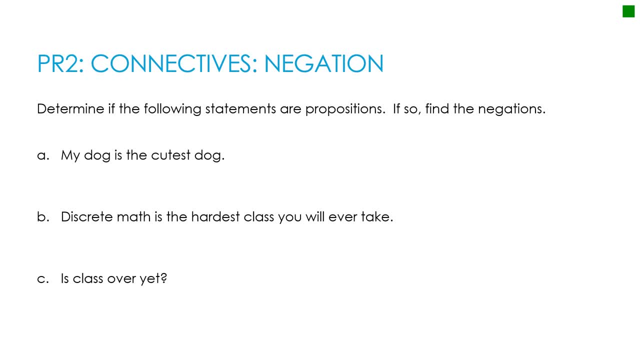 So I'd like you to press pause, try all three questions and then press play to see how you did So. for a, my dog is the cutest dog. That is certainly a true proposition, But if I were to negate it, then I would say my dog is not the cutest dog. 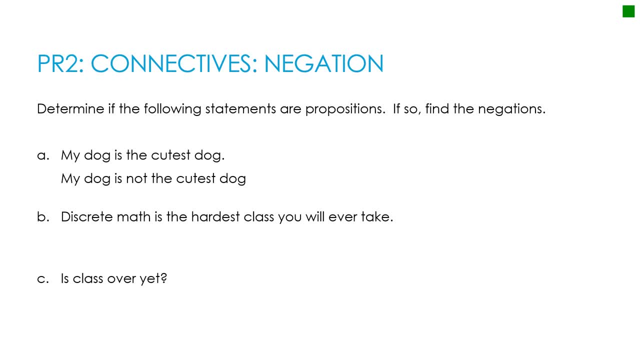 Or in quite a few of our textbooks. you would see, it is not the case that my dog is the cutest dog, But we just write things as simply as we can. Discrete math is the hardest class you will ever take. That is a proposition. 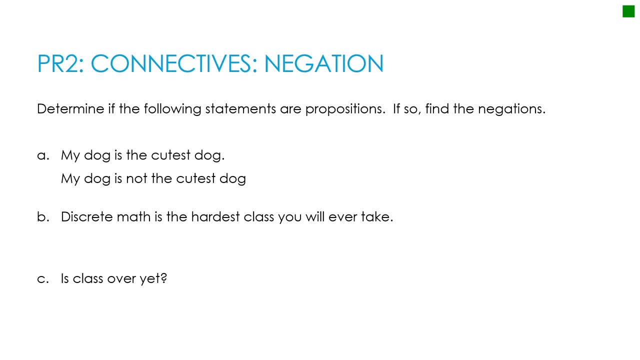 I will let you determine if that is true or false. I'm going to guess false. And the negation: discrete math is not the hardest class you will ever take. So we're just negating it, We're changing the sign. Same thing if I started out with: discrete math is not the hardest class you will ever take. 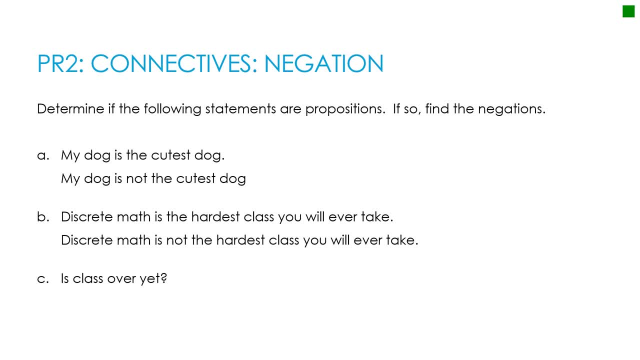 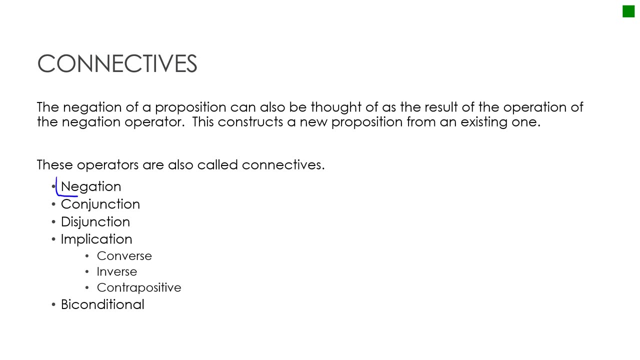 the negation would be that the discrete math is the hardest class you will ever take, And last one Is class over. yet Obviously this is not a proposition. It doesn't have a truth value. So we've had a chance to talk in a little bit of detail about the negation. 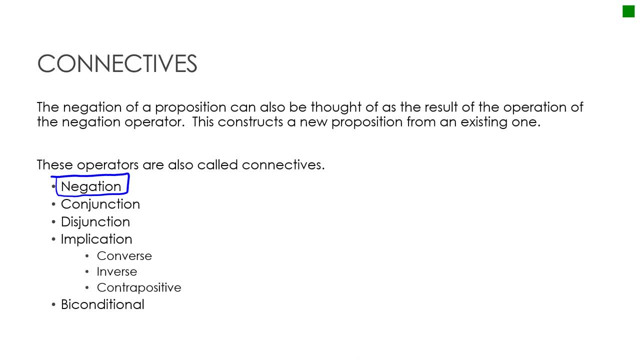 But we also have other operators that we call connectives, that are conjunctions, disjunctions, implications- as you can see there's plenty of those- and biconditionals. So over the next several slides we're going to look at each of those in detail. 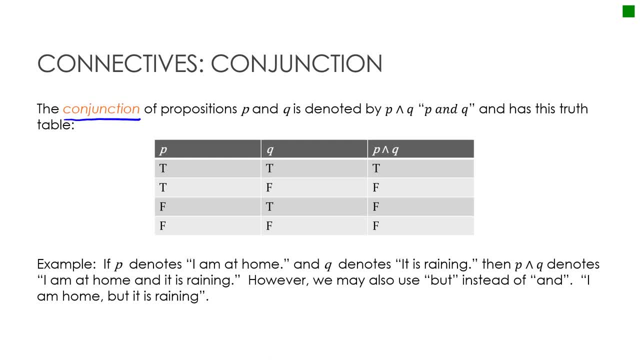 So let's take a look. Let's take a look at the conjunction. The conjunction happens between two propositions And I want you to think back to when you learned about set theory and you had A union B or you had A intersect B And it's really kind of the same idea. 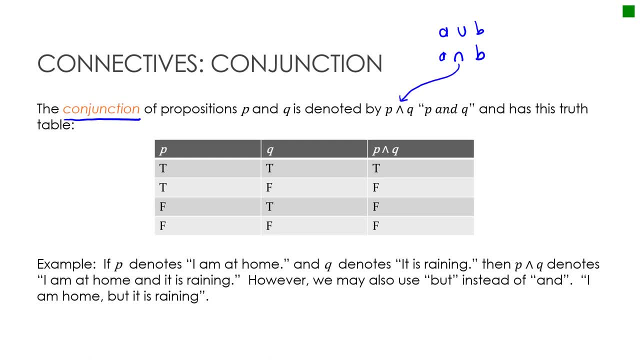 So notice this. one would kind of be like this, And whenever we looked at A, intersect B, we would always call that an and question, And that's what we're doing here. So when you see that we're going to say it: P and Q. 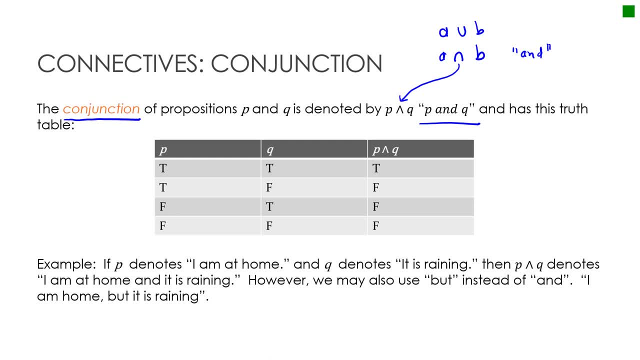 And let's take a look at this truth table, because this truth table is a little bit more complicated than that last one that we did. So in this truth table, notice that on the left here I have quite a bit more going on than before. 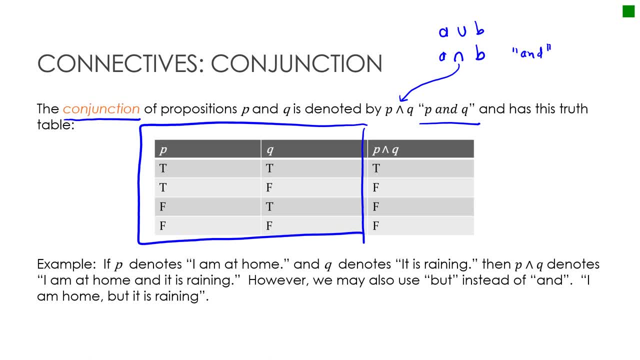 And here's why In our previous truth table I only had one proposition, So there was only one way that could happen: true or false. Now I have two propositions. So it could be that P is true and Q is true, or P is true but Q is false, or P is false but Q is true, or P is false and Q is false. 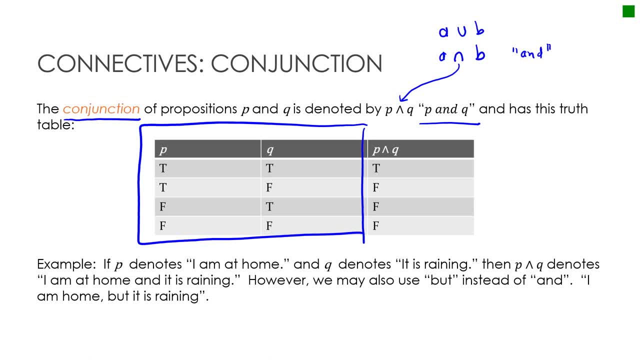 So, in terms of the result over here, which is P and Q, what we're looking at is for both of them to be true. So, as we can see in row one here, P is true and Q is false. P is true and Q is true. 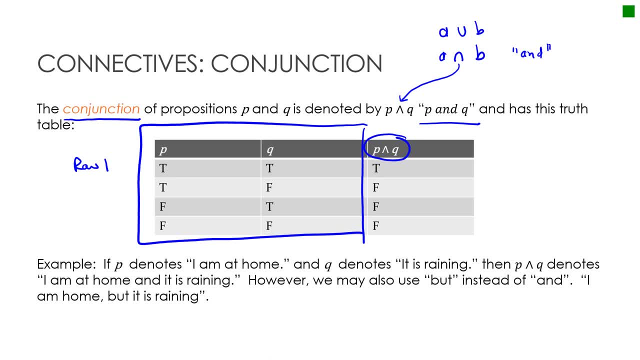 And so that has a true conjunction of the two true propositions. The others are all false because they both have to be true in order for the conjunction of them to be true, And obviously we can see that that's not the case for any of the other rows. 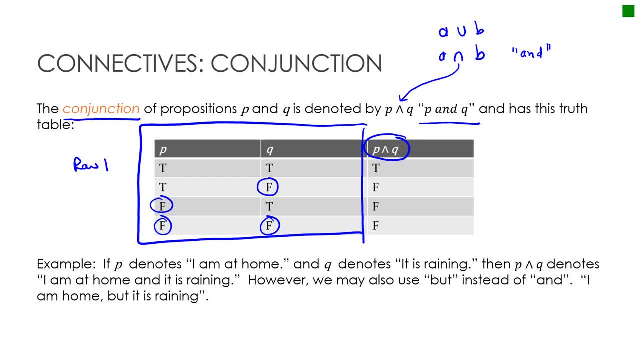 So, as an example, let's say P denotes I am at home, Q denotes it is raining. Those are both propositions. They both have truth values. We don't know what the truth values are, but it doesn't matter. Then P and Q denotes I am home and it is raining. 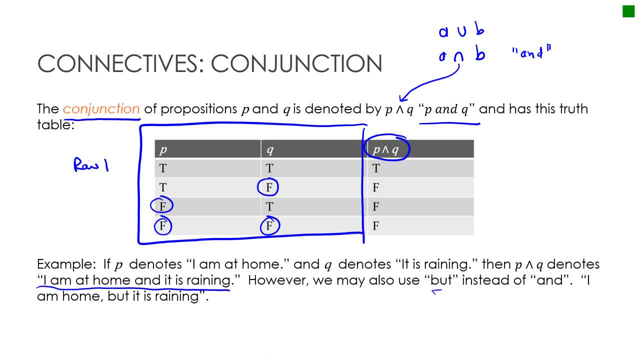 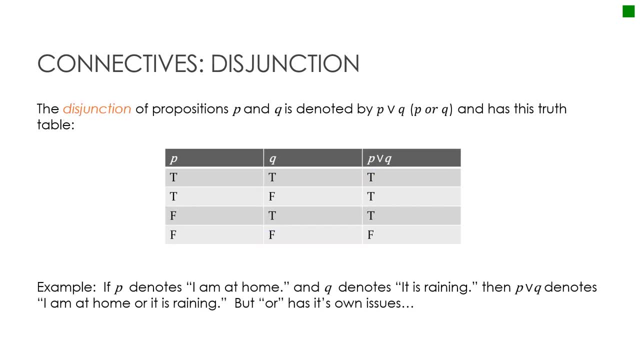 I typically stick with this one. I know some people can go into the buts, but just don't do it. It just makes it more complicated. So now let's take a look at disjunctions. The disjunction of a proposition. 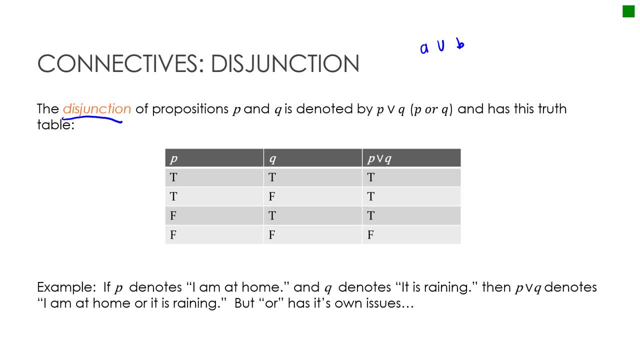 Again, I want you to think about that: A union, B- same kind of idea. We're saying, hey, we're satisfied if either A or B is true. Same idea. here We're saying P or Q, So we're using that word, or when we're saying it aloud: 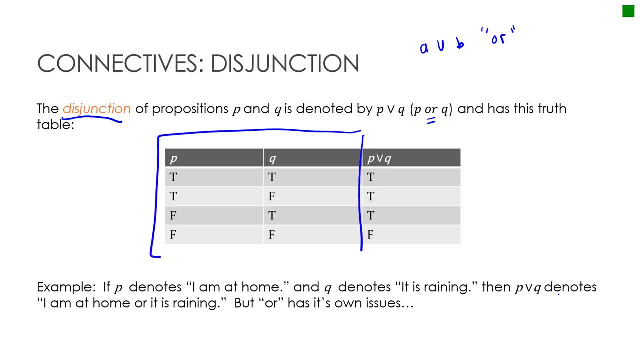 And again, let's take a look at the truth table. I want you to notice, on the left hand side, this looks exactly like the truth table for P and Q Because, again, these are the four different possibilities for the two propositions of P and Q. 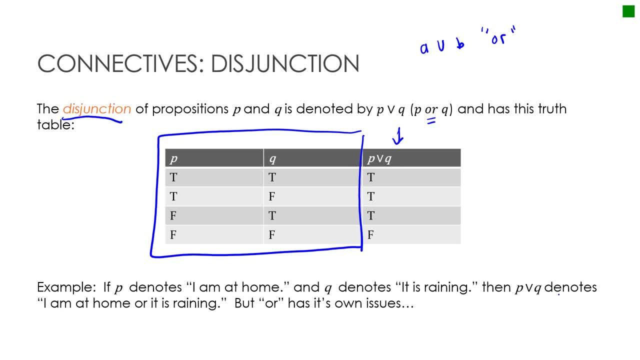 Now this column, Obviously, is different, because now we're saying, hey, if one or the other is true, then we're satisfied And the whole statement, the whole disjunction is true. So notice here: They're both true, which means yes, at least one of them is true. 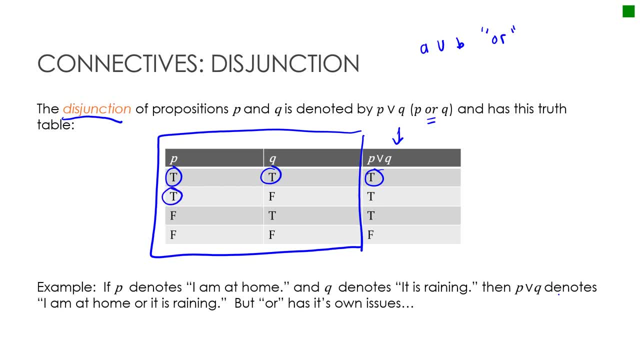 On my second row, P is true, So it really doesn't matter if Q is because we've got at least one that is true. On my third row, Q is true And therefore The whole disjunction Is true. And then notice here: 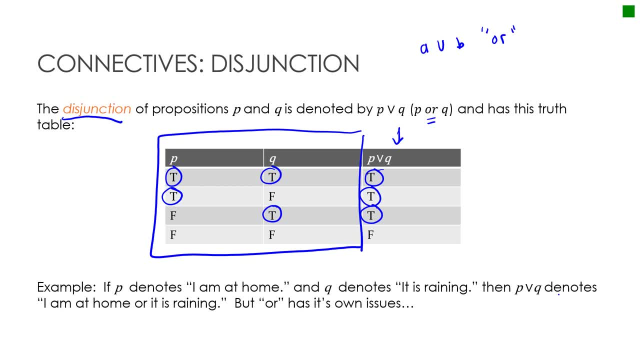 There are no trues. P is false, Q is false. Therefore, P or Q is false. So again for an example, we're still using at home and raining, Then P or Q denotes I am at home or it is raining. 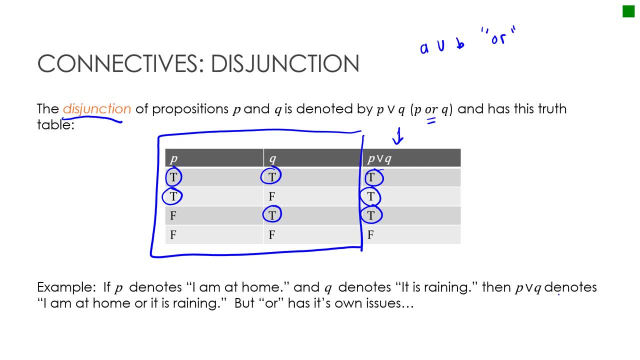 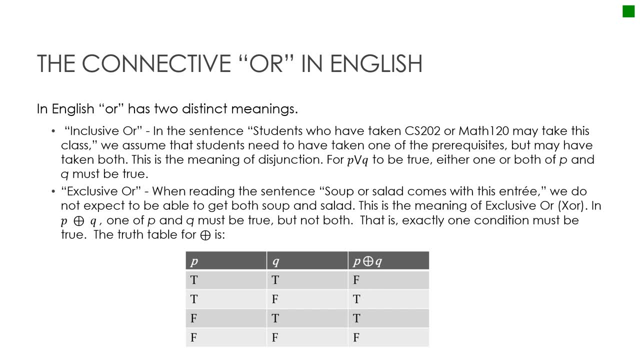 And again or does have its own issues And we're going to talk about those. So we've got this or in English, and then we have or mathematically. So there's the inclusive or In a sentence. Students who have taken CS 202 or math 120 may take this class. 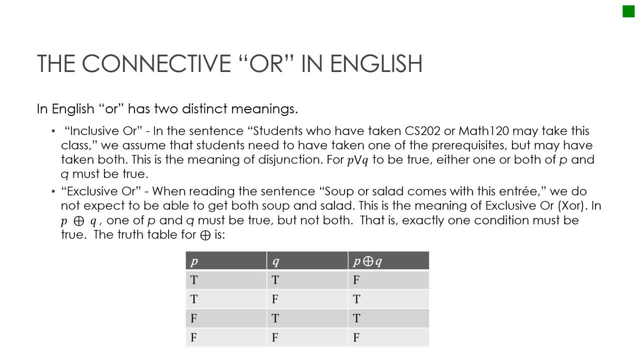 So we can assume that students have to have taken one of the prerequisites, but they might have been able to take both, And that is what we're looking at in a disjunction. Okay, One or both needs to be true. However, when we're reading a sentence, soup or salad comes with the entree. 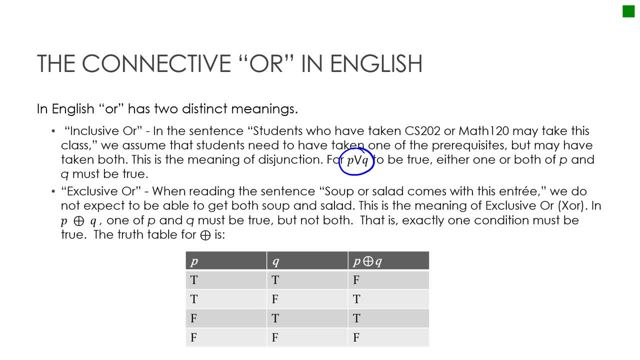 Unfortunately I can't have both soup and salad. I have to choose one or the other. So that's exclusive, or- And that is the symbol that we use, And we say that X or So again you can see the truth table here. 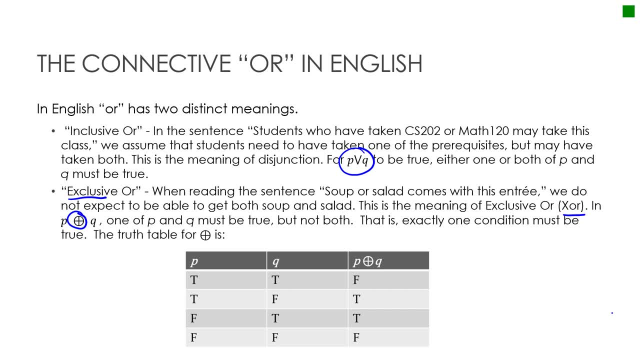 This one is saying, essentially, that only one of them can be true. So notice here: one is true, And so I get a value of true. One is true, So I get a value of true, But this one that was true before is now false because only one of those two can be true. 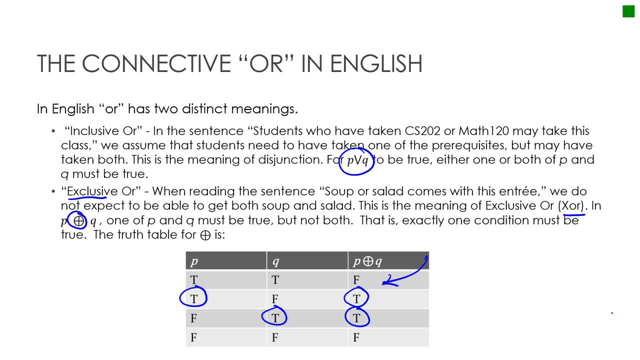 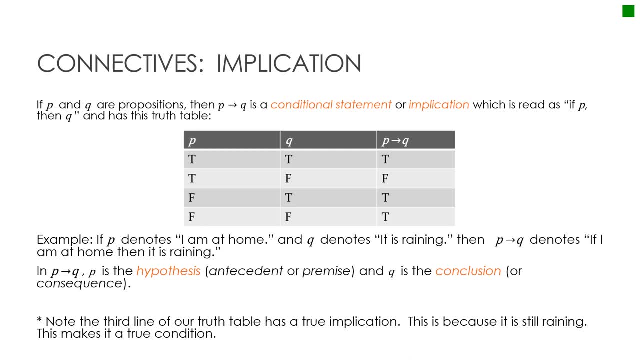 So hopefully that makes sense. The difference between or and X, or The next one we're going to talk about, is an implication, And an implication is obviously, when you think of the word implies. one implies the other. This one gets a little bit trickier with the truth table because we're basically saying if P, then Q. 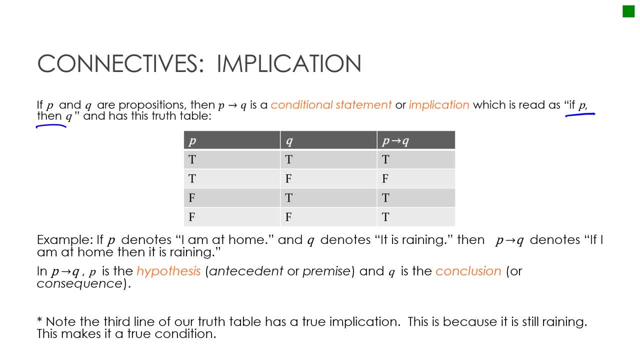 So again, this left side. this is nothing new, This is the same that we've seen before, But the if P then Q. Most people understand this one And this one quite easily, because if P is true, then Q is true. 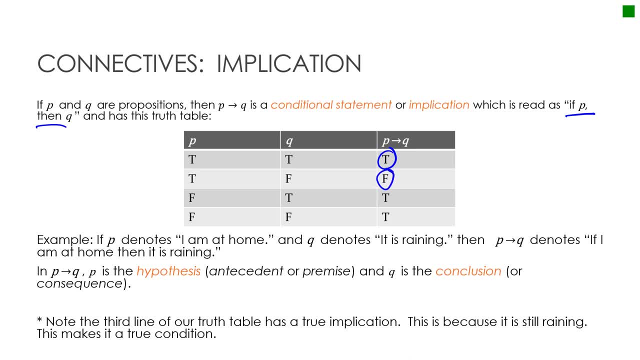 And most people understand this one quite easily, because if P is true, then Q is false. Obviously we want it to be true And therefore the if P, then Q is false, because we're saying if P is true, then Q must be true. 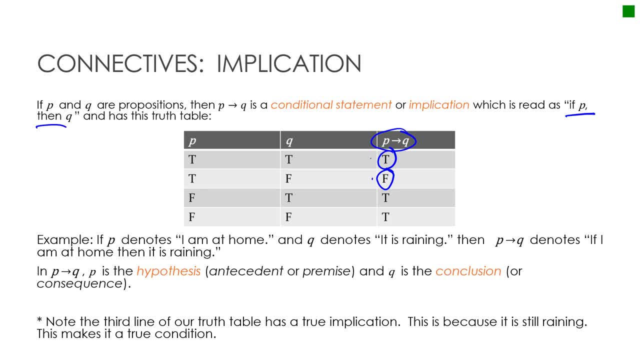 So this one is true, This one is false. But now let's look at the next two. So we're saying: if P is false, Then what Do we care? what happens with Q? Well, no, not necessarily, because our conditional statement says: if P is true, then Q is true. 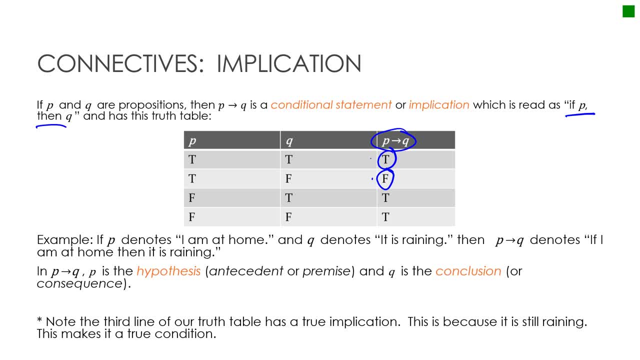 It doesn't say what happens if P is false. So, since P is false, Q is true, Sure If it's false, Sure, Because P was false on both of those. So again example: I'm at home and Q is, it's raining. 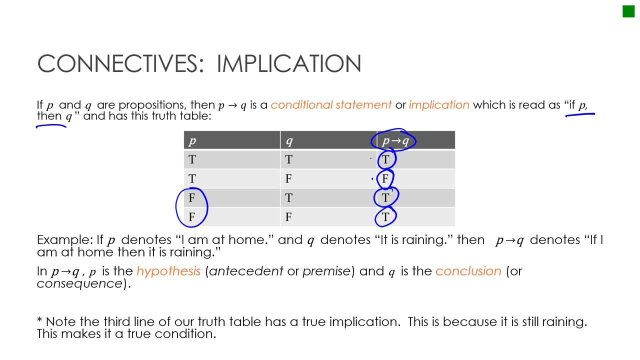 Then if P, then Q says: if I'm at home, then it is raining. So how does this work when we're looking at the false ones? If I am not home, Well, then it could be raining, or it could not be raining, because it doesn't say anything about that in terms of, essentially, this is directional. 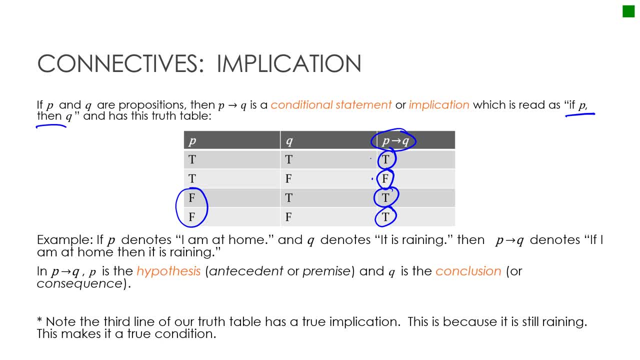 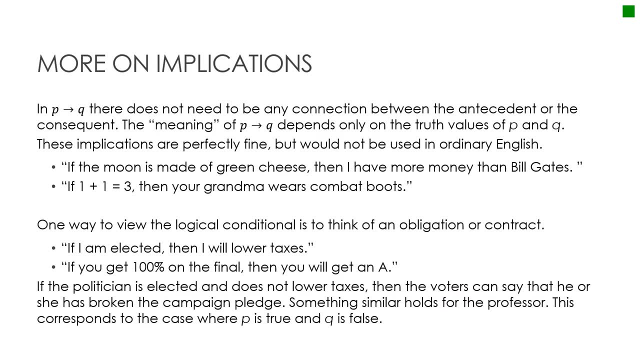 So hopefully that makes sense, because there's going to be another one that is not directional And it's very important to keep those two separate. So a little bit more on implications. Keep in mind that These implications- the if P, then Q- is all just based on truth values. 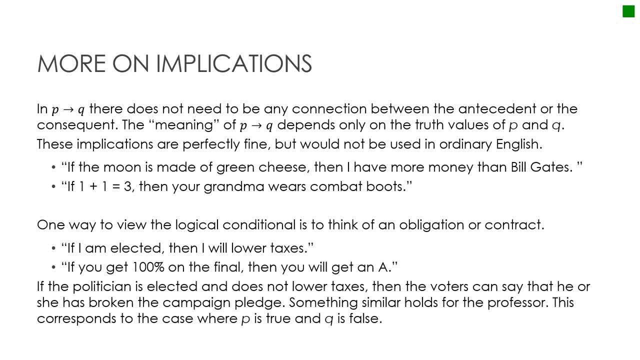 It doesn't necessarily need to make logical sense in terms of real life. So if I've got, if the moon is made of green cheese, so the moon is made of green cheese is P, Then I have more money than Bill Gates would be. Q. 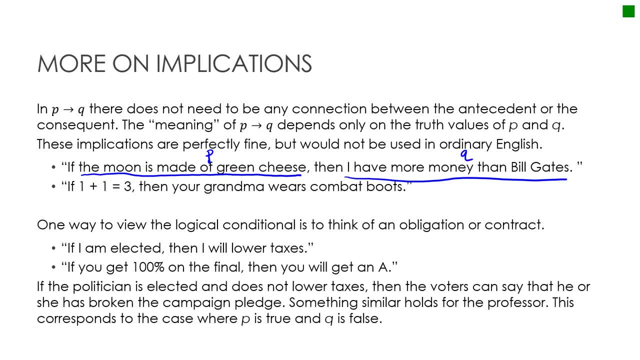 So this doesn't make any sense, Obviously, and whether or not the moon is made of green cheese in real life would have nothing to do with whether or not you have more money than Bill Gates. So we're looking just at truth values. If this is true, then this is true. 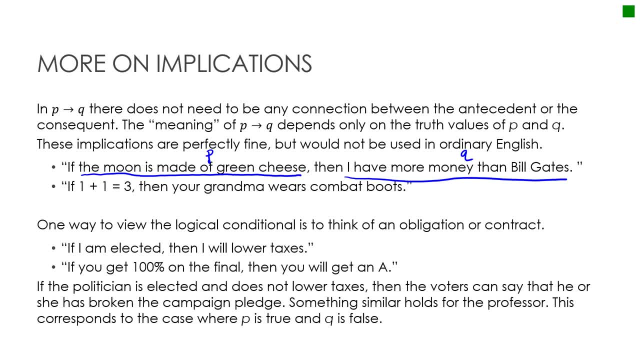 If one plus one equals three, then your grandma wears combat boots. Again, those two things don't? It's hilarious. I want to see my grandma wearing combat boots, but it doesn't need to make sense. The two, the P and the Q, don't necessarily make sense. 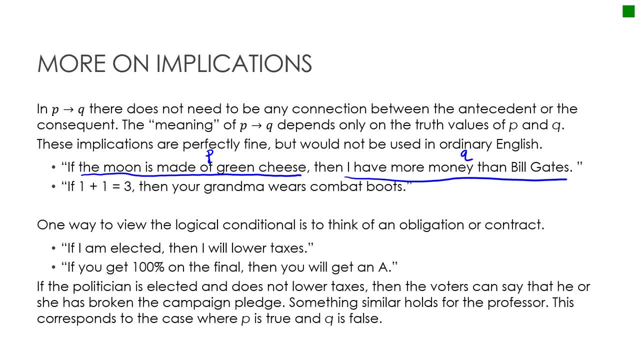 You don't necessarily need to be talking about the same thing, But obviously we have logical conditionals, and logical conditionals is where they actually sort of are related to one another. If I'm elected, then I will lower taxes. If you get 100% on the final, then you will get an A in the class. 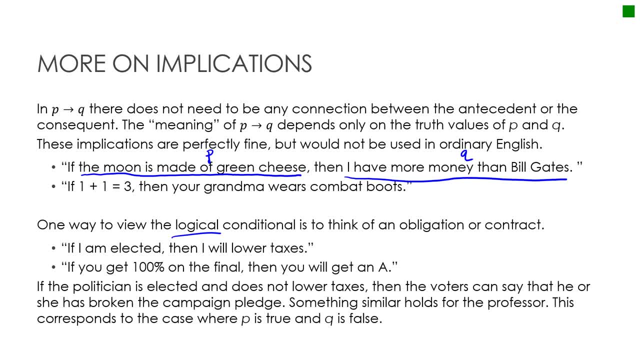 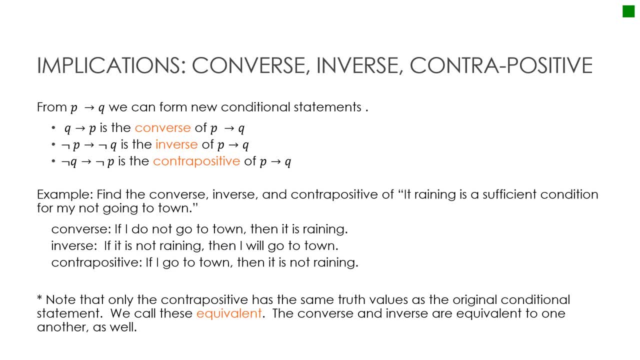 So those are conditionals that are, you know, based on- still based on truth, values, but maybe go together a little bit better. So let's take a look now at some of the Different implications that we have from an implication: the converse, the inverse and the contrapositive. 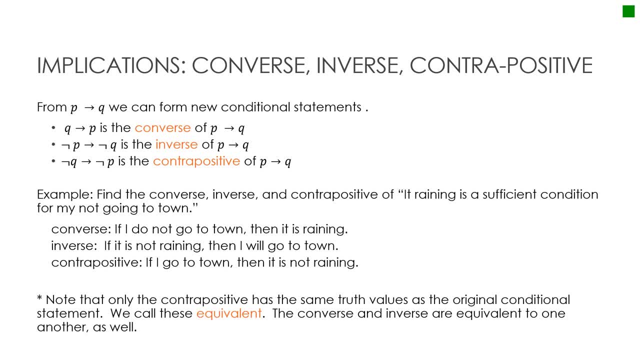 So the converse is essentially us switching the order of the two. If Q, then P. Now, obviously this is probably not going to have the same truth value or truth table as your original implication. Now let's look at the inverse. Inverse is: if not P, then not Q. 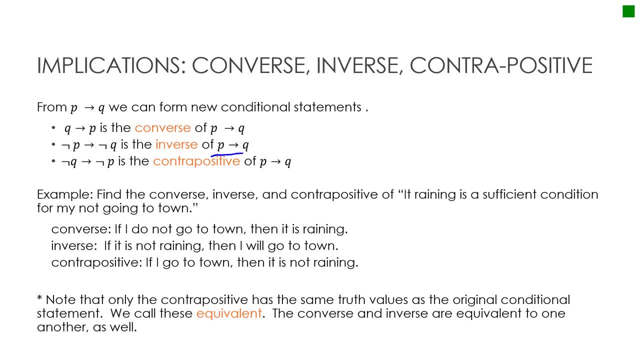 So notice, it's the original order- that I have P and Q And I'm negating each. So that's what happens in an inverse: is we negate each, So this one is switch order, This one is negate, And then the contrapositive is basically putting it all together. 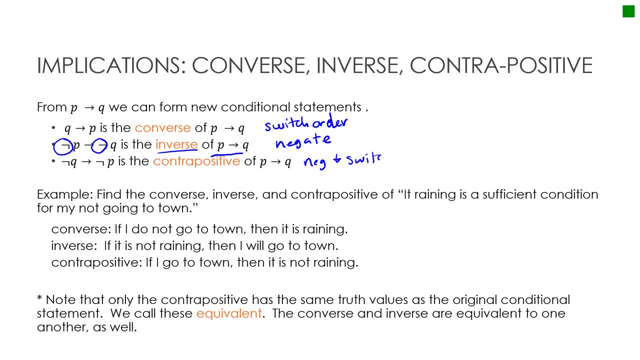 I'm negating and switching. So if not Q, then not P. Now what's important to understand is That truth Table that we would make for the original implication Would be exactly the same for the original implication and the contrapositive. 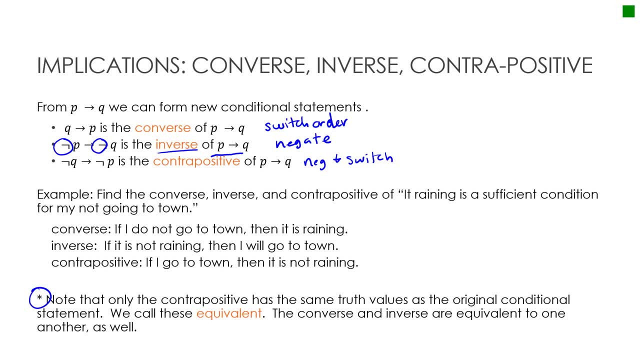 It would not be the same for either Neither the converse nor the inverse. So, for example, If I'm looking for the converse, inverse and contrapositive of It is raining- as a sufficient condition for my not going to town- And you might look at this and say, well, what does that mean? 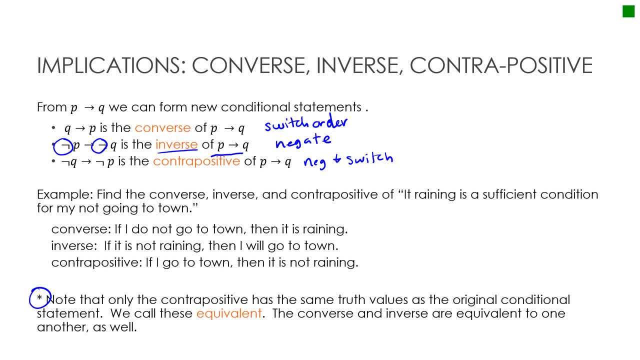 So it's okay, Before you try to find Any of the other implications, to write it in a way that makes more sense to you. If it is raining And this is P, Then I will not Go to Town. That's Q. 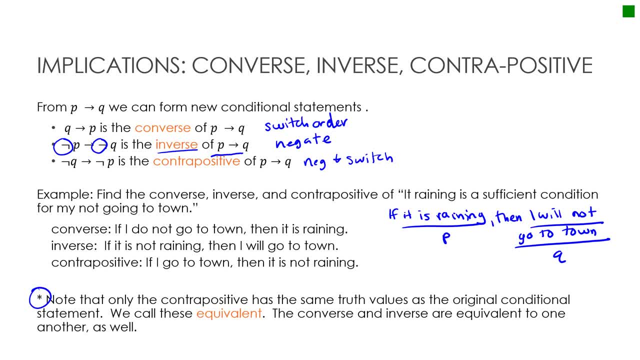 So now that I have it in a way that makes sense to me, I'm going to look at the converse, which is switching the order. So if I do not go to town, then it is raining, So all I did was switch the order of P and Q. 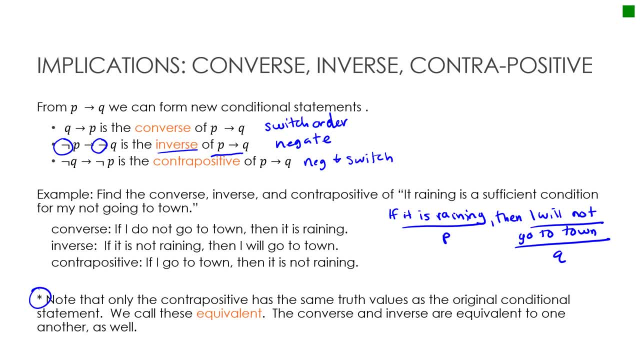 Inverse. I'm going to keep them in the right order, but I'm going to change the. The values I'm going to get negate each. So if it is not raining, Then I will go to town. So this one. 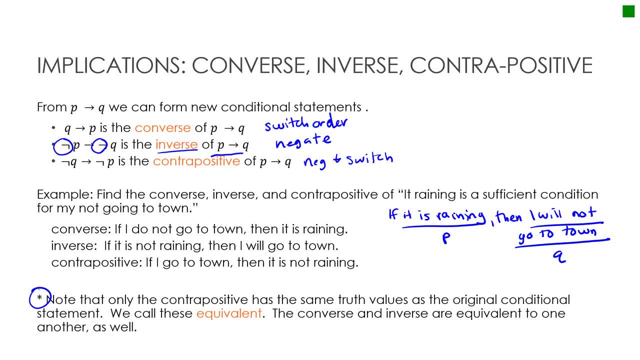 I changed to not. this one already was not, So I changed to I will And the contrapositive. I switched the order and I negate each. So if I go to town Then it is not raining. Okay, Now I have one of those for you to try. 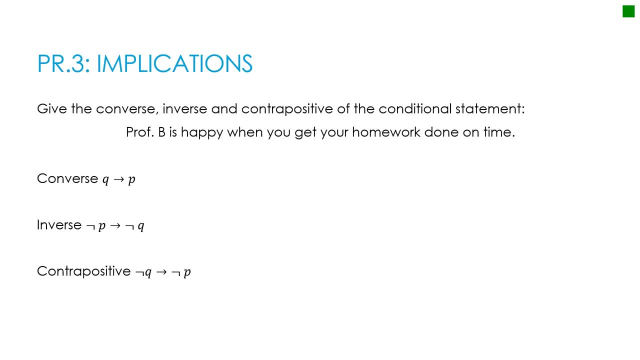 So I've given you the statement. Professor B is happy when you get your homework done on time. Now this one might mess with your head a little bit. So before you try to do the converse, inverse and contrapositive, At least while you're practicing. 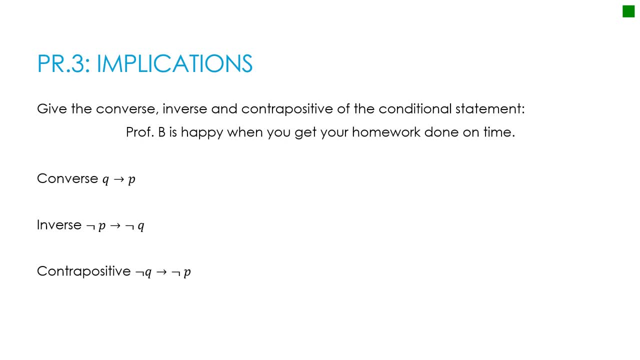 I suggest writing this and if then form So it's very clear What is P and what is Q, And then writing the converse, inverse and contrapositive are actually quite easy. So Press pause, Rewrite The original implication And then write each of the other three implications. 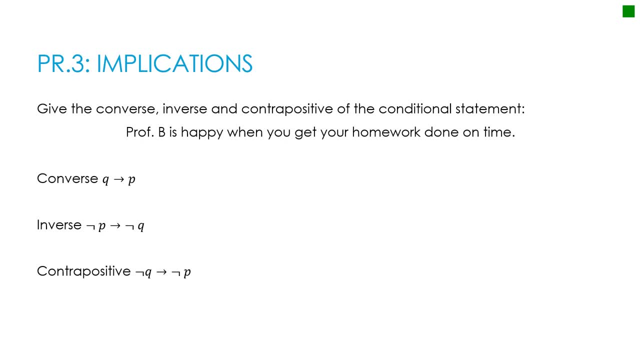 And then press play to see how you did So. again, The first thing I'm going to do here Is: I definitely want to do a rewrite, And the rewrite is: if you get your homework done on time, Then Professor B is happy. 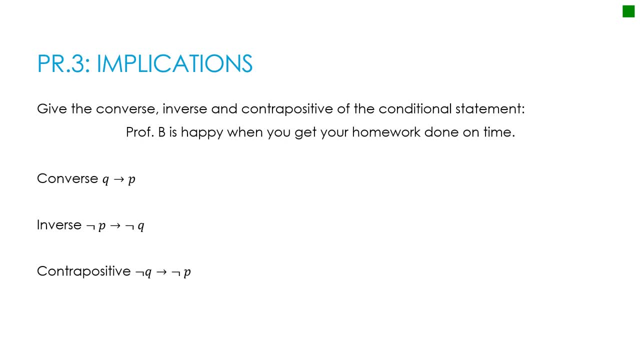 Now a lot of people struggle with that Because, Look, This happens first in my sentence. But you really have to think about Which Property Is Happy. When you get your homework done on time, Then Professor B is happy. 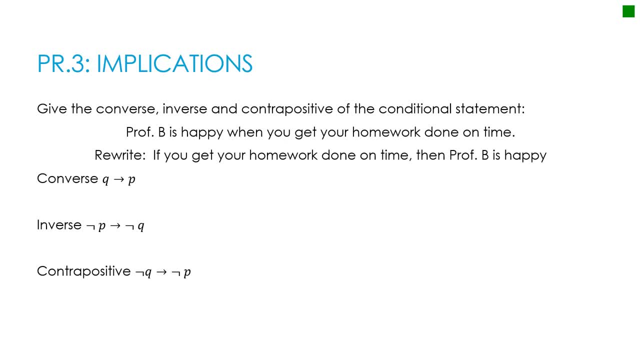 Now a lot of people struggle with that Because, Look, This happens first in my sentence. But you really have to think about Which Property Is Happy When you get your homework done on time, Which means This has to happen first. 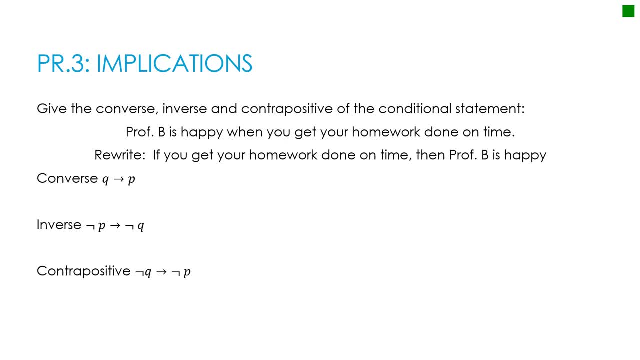 You have to get your homework done on time In order for me to be happy. It's kind of sad, But You get the idea. So now let's look at the Converse. Well, Before I do that, You get your homework done on time. 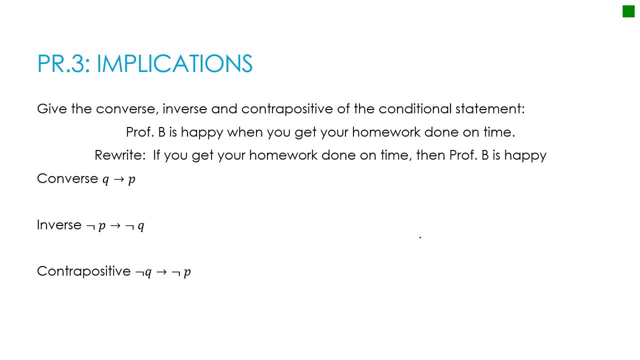 Is P And Professor B is happy Is Q? So let's take a look. The converse Is Happy When You Get Your Homework Done On Time, If Professor B Is. 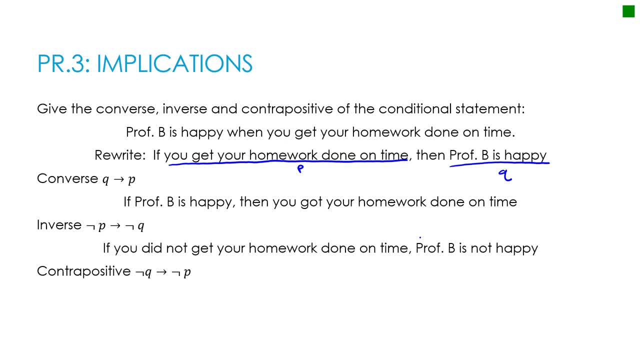 Happy Then You Got Your Homework Done On Time. The inverse- Remember I'm Negating: If You Did Not Get Your Homework Done On Time And 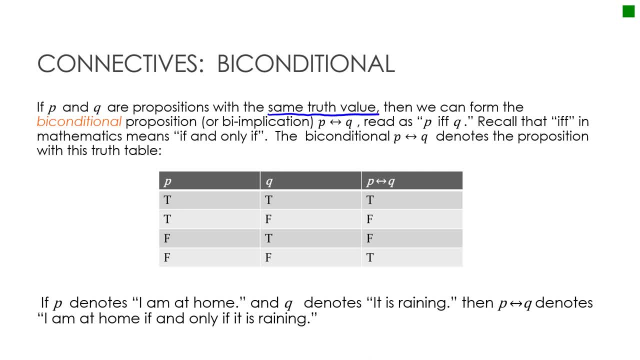 You Get Your Homework Done. You Get Your Homework. Get Your Homework Done. John Is Happy When You Get Your Homework On Time, If You Get. 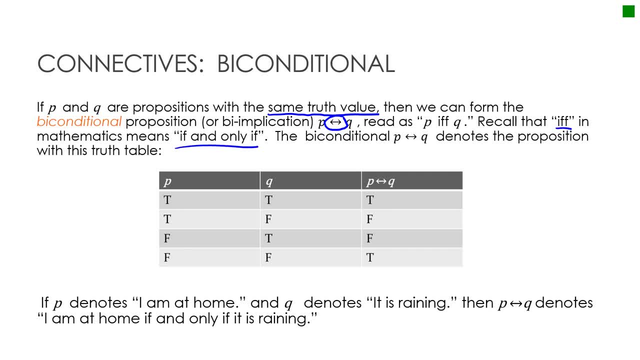 Your Homework. Then, and only if So, the biconditional. if p, then q has the truth table right here, and so remember, this is only going to be true when p and q both have the same truth value. So here p and q are. 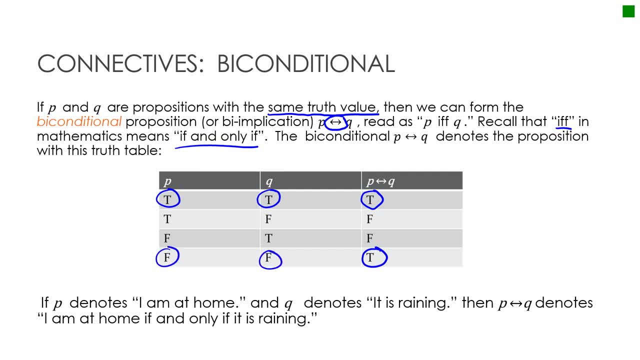 both true, so it's true. Here p and q are both false, so it's true. Notice the others where p and q have a different truth value result in a false result on the biconditional statement of the truth table. So if p denotes I am home and q denotes it is raining, then p if, and only if, q. 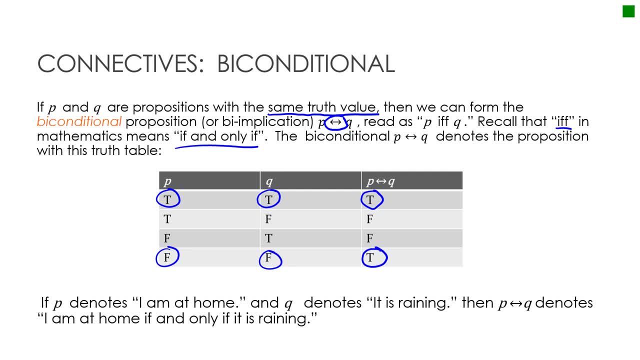 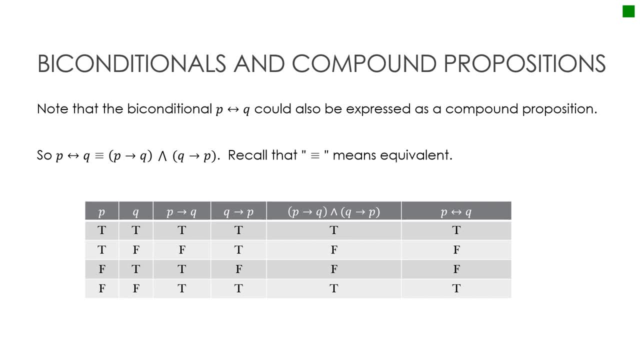 denotes I am at home if, and only if, it is raining. We haven't looked much at compound propositions yet, although that will obviously be a huge part of what we study as we're looking at truth tables and conditionals etc. But notice that the same way that I could write p if and 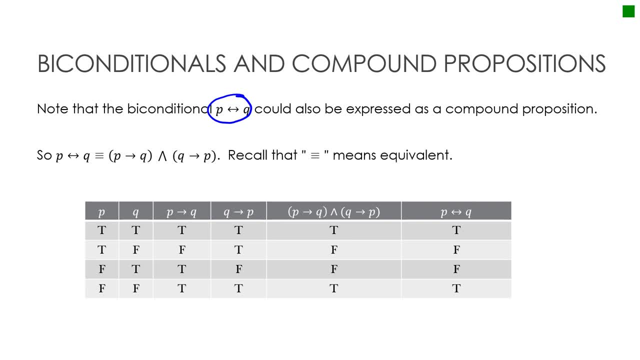 only if q. I can write it in another way and that other way. so notice, here I'm saying p if, and only if, q is equivalent to, and then I'm saying: if p, then q, and then what's this one mean? 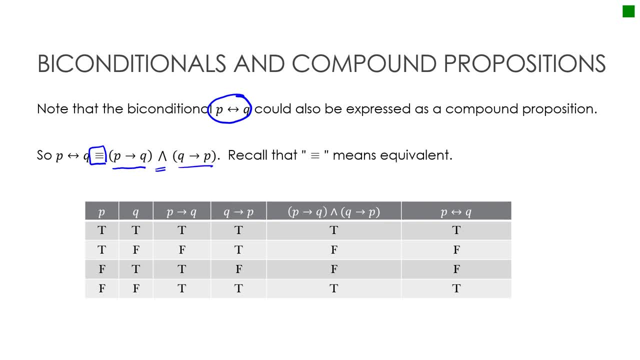 and if q then p. So essentially I'm saying these two things are the same. So if p, then q. we already found these values of the truth table on the previous slide, but now let's take a look at the truth table. that would help us come up with the truth values for this compound proposition. 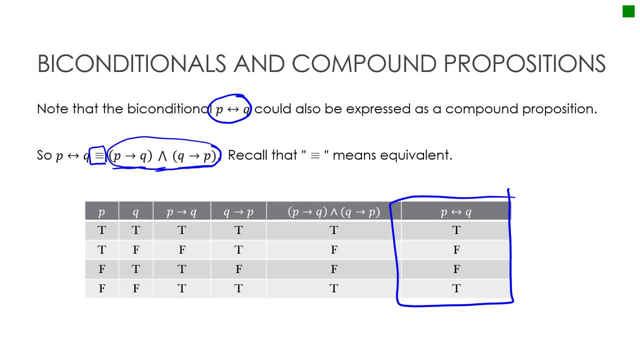 So again, this first row is just showing the different values that p and q. sorry, the first two columns are showing the different values that p and q can have: True, true, true, false, false, true, false, false. And then we start actually coming up with the values. 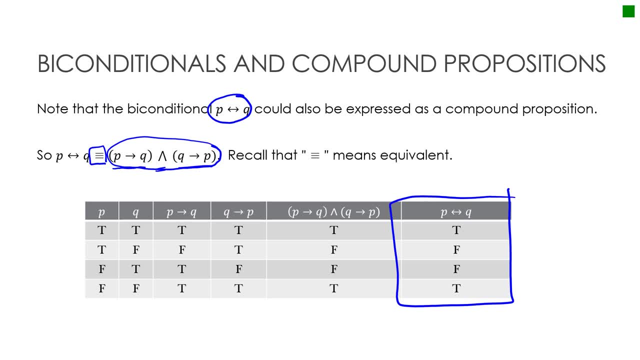 so these are things that we would like to see. So if p and q are equivalent to- and then I'm going to have to then figure out- So the first one says: if p, then q. so obviously this one is true, because these values are both true. This one is false because this is: if true, then false. 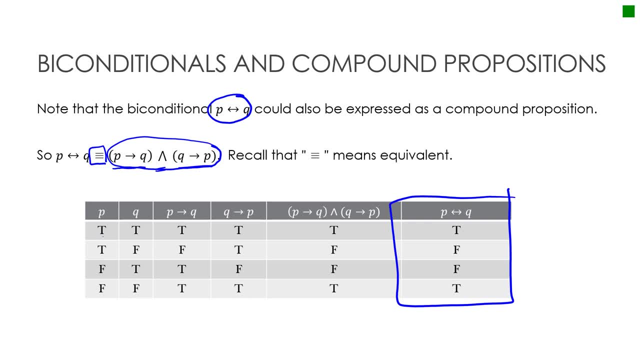 And then remember, these are those two tricky ones, because p is false and so, because it's one directional, we only care about it when p is true. So now let's look at the same thing. We're looking at: if q, then p. So if q, then p, and then I'm going to have to figure out. 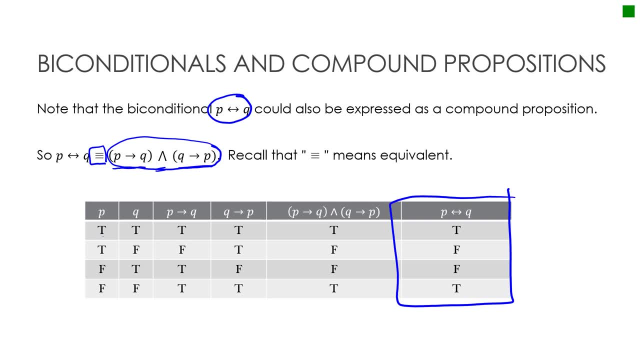 if q, then p would be true, then true, This one would be true as well, again, because q is false. This one would be false because if true, then false doesn't work. And then this one would be true because that first value in the implication is false. So now that brings us to this. 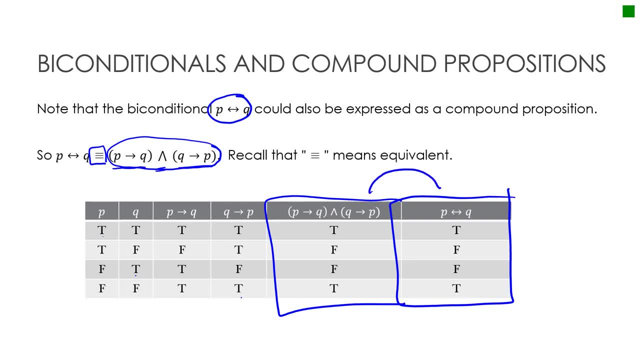 column right here And this column right here. what we're saying is these two should have equivalent truth values. So let's take a look at why this is. This says: if p then q and if q then p. both have to be true. 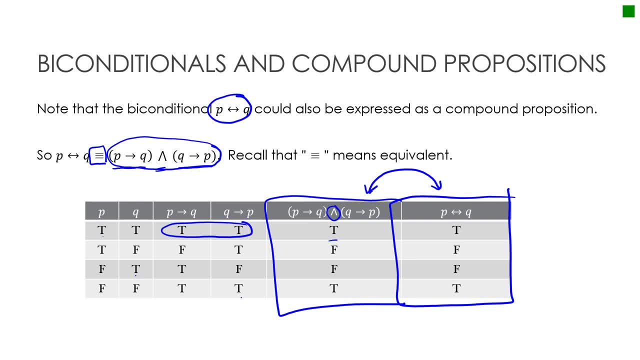 So this is true and notice, I've written true here. This one does not work because they're not both true. This one does not work because they're both not true. This one, they are both true and therefore I get true, false, false. 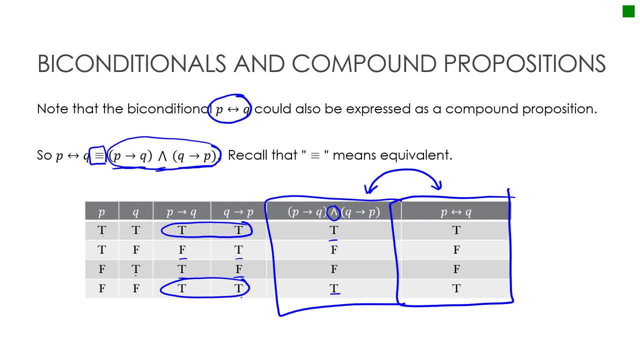 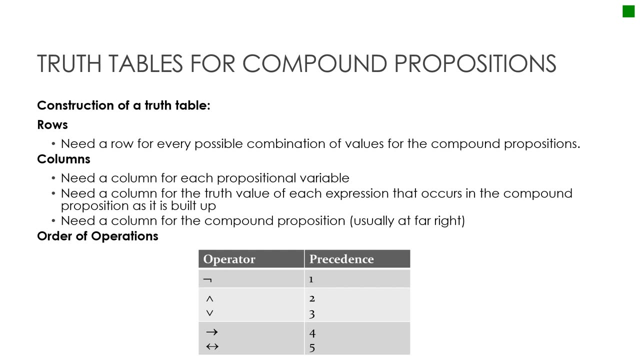 true, and that happens to be the exact same thing I had on the other screen. So I just wanted to point out to you that these are two equivalent things, So one of them written as a compound proposition, one of them written as a biconditional. So we haven't really talked. 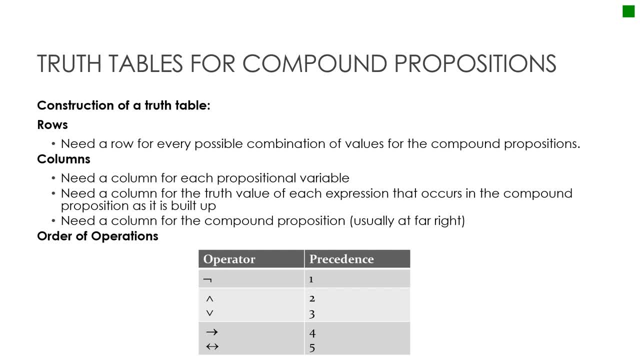 explicitly about how to create a truth table, though we've seen quite a few examples, So I really wanted to go through how to create a truth table or the process that we go through. So we already kind of knew that we would need a row for every possible combination. 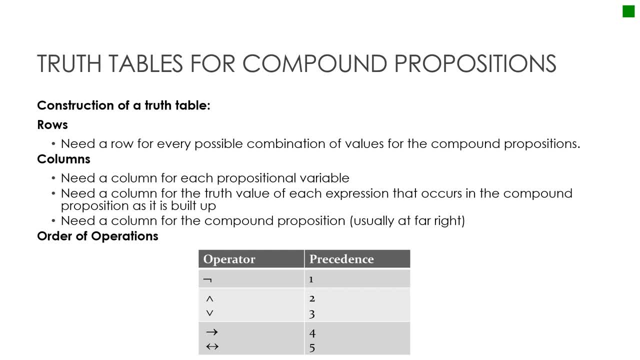 of values for the compound propositions. So let's say I was using p and q, which is two of them. Then I know the possible combinations are true, true, true, false, false, true and false, false. So essentially four rows. Now if I threw an r in here as well, well then I would need a row for r. 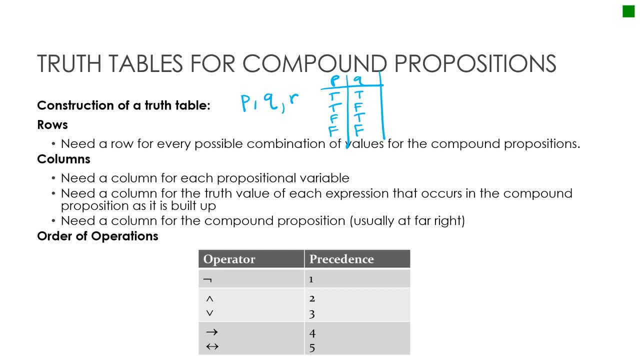 and four rows isn't going to do it anymore, because I could have r as being true for each of those combinations, or I could have r as being false for each of those combinations, and therefore I would need eight total rows. So what we're looking at here, then, is essentially having two to 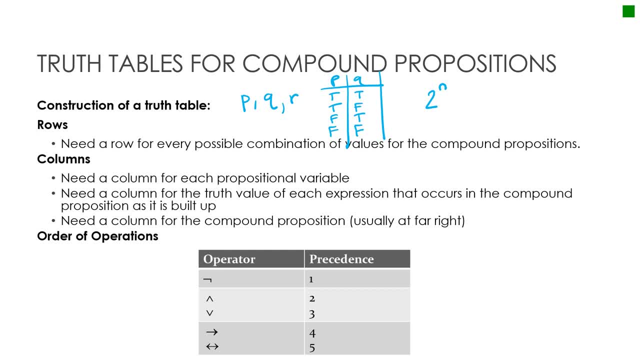 the n rows, where n is the number of propositions. So here, where I had just p q, that meant four rows. If I had p, q, r or three propositions, that was eight rows. then in terms of columns, let's say we are looking to. 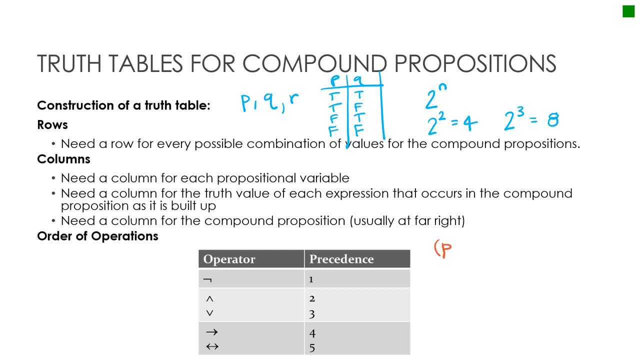 create a truth table for P and Q or R and not P. so we've got a lot going on here and what I would need is: I would need a column for P and for Q and for R. I would need a column for P and Q. I would need a column for, not P, because 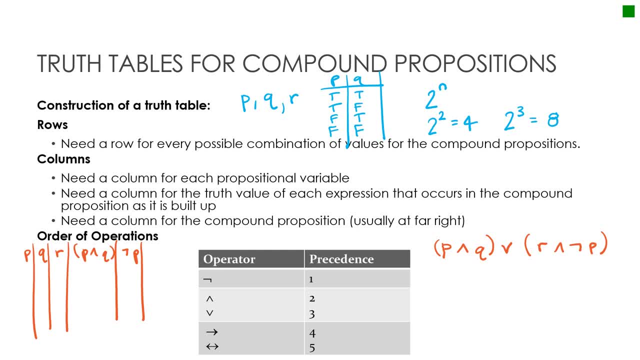 not P is used over here, and then I would need a column for R and not P. and then of course I'm out of room, but my final column would be everything put together, P and Q or R and not P. so here I would have one, two, three, four, five, six, seven columns. also, it's important to understand what 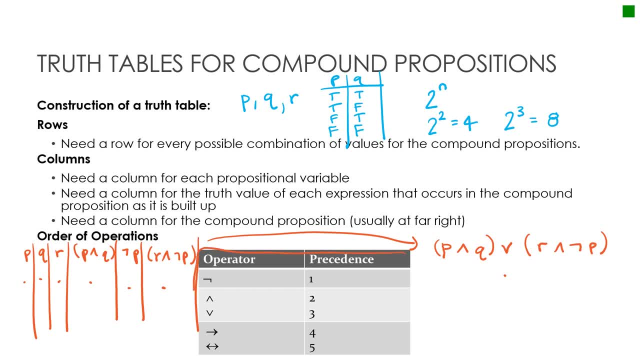 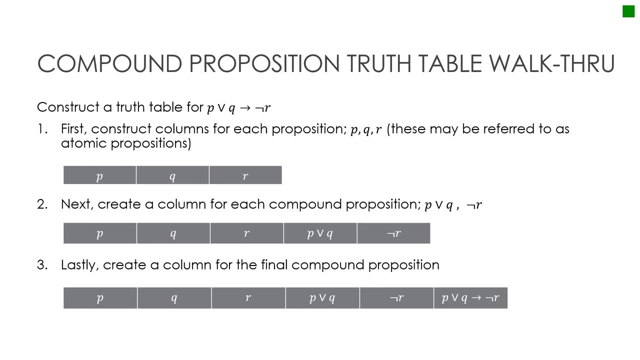 the order of operations is, or order of precedence is, and here we can see which order we would go in in terms of finding a, not finding an and then an, or finding an if, then, or finding an if and only if. so here's a compound proposition and we're gonna. 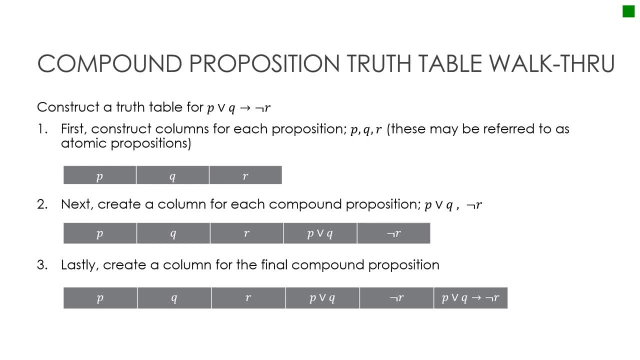 create this truth table together and we're gonna do it really kind of slowly, step by step by step, but essentially here is the compound proposition that we are going to create a truth table for. so I know right off the bat that I'm going to need a column for P and Q and R and I know that I'm going to have eight rows. 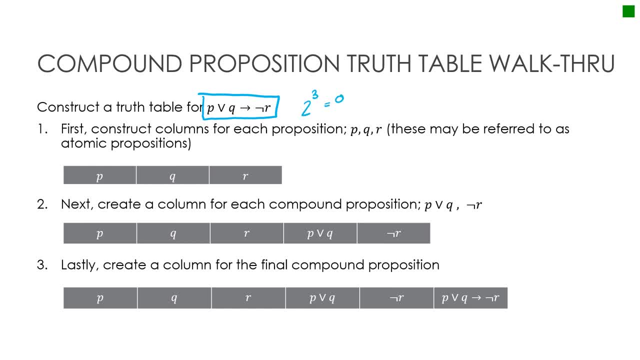 because it's two to the third, which is eight, remember? the three is: how many different propositions do I have? and two is because each of those values has, true and false, two different options. next, we're going to create a column for each compound proposition. so notice, here I've got a. 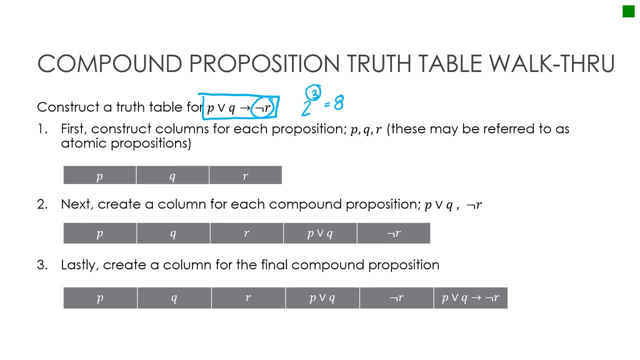 not R. and a lot of people are like, well, do I really need to put not R? yes, you do. you really need to put not R, even though it's just the opposite value of whatever you have in R. and then our another one is P or Q, and then notice, the one at the very end is our final compound. 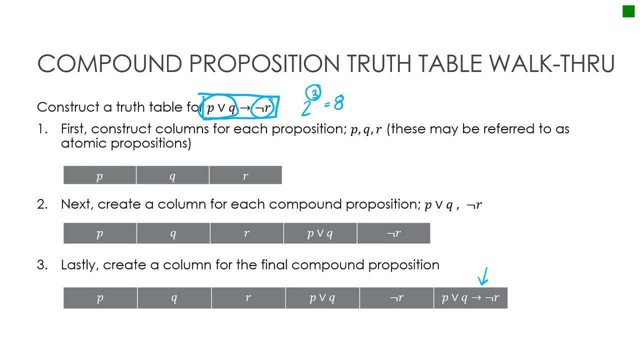 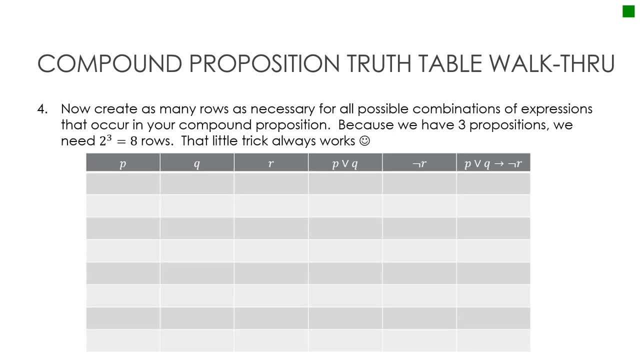 proposition, which is, if P or Q, then not R. so that's our final solution, our final thing that we need. again, remember we talked about two to the third or eight rows. so now we have as many rows that are necessary and we have all the combinations that we need. 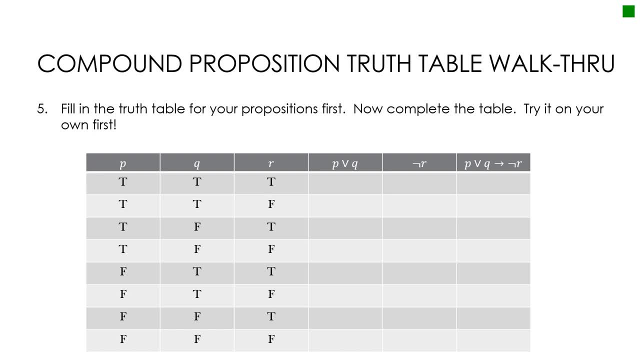 and now we're going to fill in the truth table for your proportions first. so I haven't had to do any thinking yet. I haven't had to really look at anything. I've said, hey, I need for these three, I need all of the different combinations that could happen with P, Q and R in terms of truth values. so I've got true. 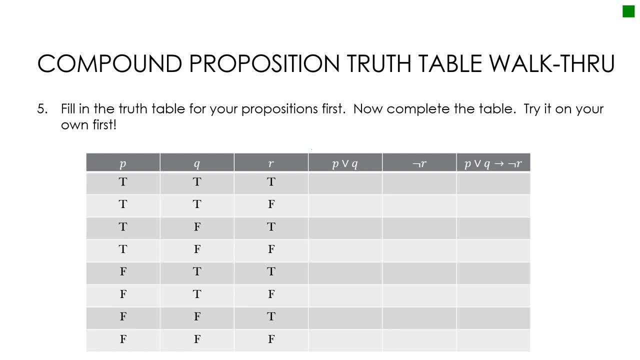 true, true, true, true, false, true, false, true, true, false, false, etc. different people have different strategies for how to keep track and make sure they all get there. I tend to just try to keep it as simple as possible. notice what happens. here is my first column. I've got four trues and 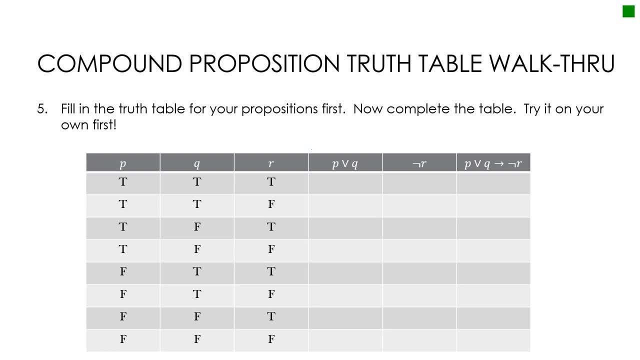 four falses, and then I alternate: two trues, two falses, two trues, two falses. you get the idea. so, before we continue, what I would like for you to do is to press pause from right here and see if you're able to complete the rest of this. 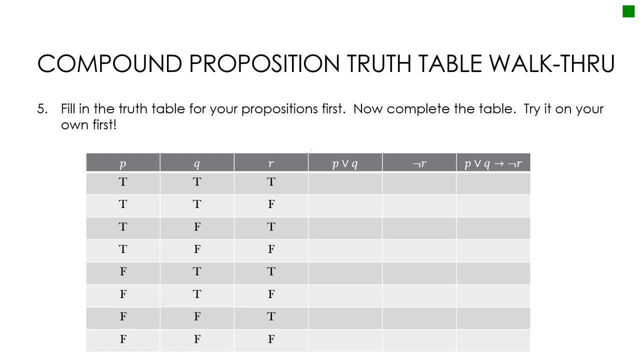 truth table on your own. so let's take a look at the values again. if you hadn't paused already, go ahead and do that, but let's take a look at the values we should have in our truth table. this column says P or Q, so essentially I'm 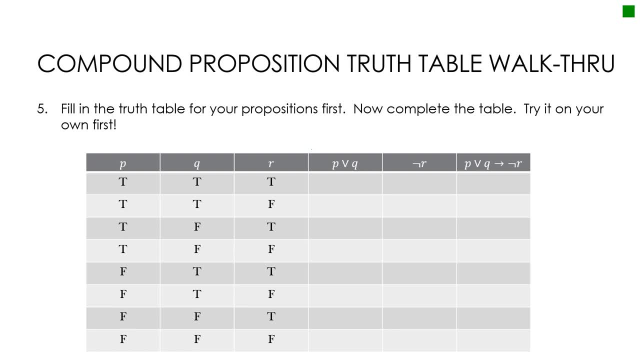 saying: if P is true or Q is true, then I'm satisfied. so here I've got true. true, that means this is true. same thing here. this is true. my third row of: again P is true. it doesn't really matter if Q is, because all I need is one of. 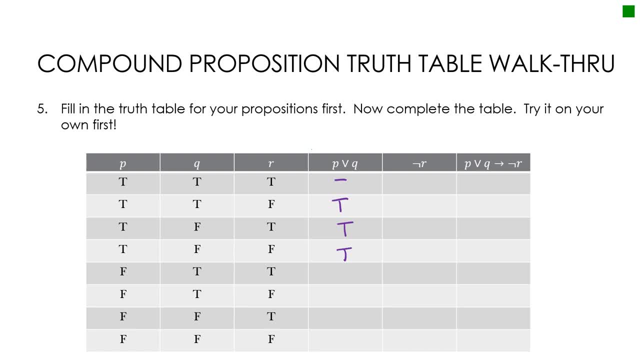 them to be true. same thing here. this is true because P is true. my next column is true because true. Q is true. now, I'm looking at these two and I've got at least one. true. I'm looking at these two and I don't. I'm looking at these two and 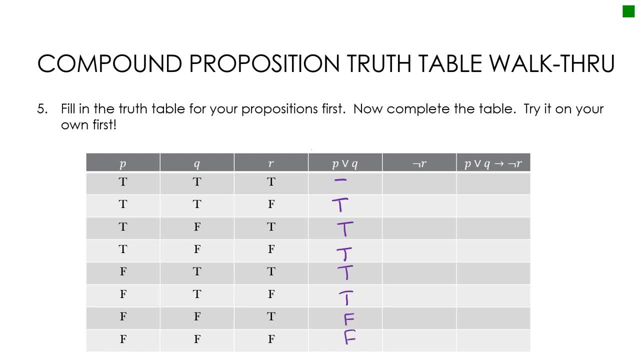 I don't. so that's that first column. now I'm gonna erase all of my marks, so it doesn't get crazy. and now let's take a look at. not are obviously this one's super duper easy because it's whatever's in our. I'm just putting the opposite thing, so true. 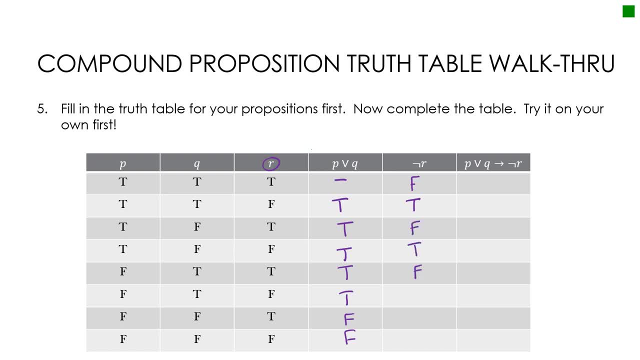 becomes false, false becomes true, true becomes false, false becomes true, true becomes false, false becomes true. and now for my final solution, which is we're saying essentially this: P or Q, or if P or Q is true, so now let's take a look at: or Q, then not R. So, with P or Q being true, then not R needs to be true, So this one has to be. 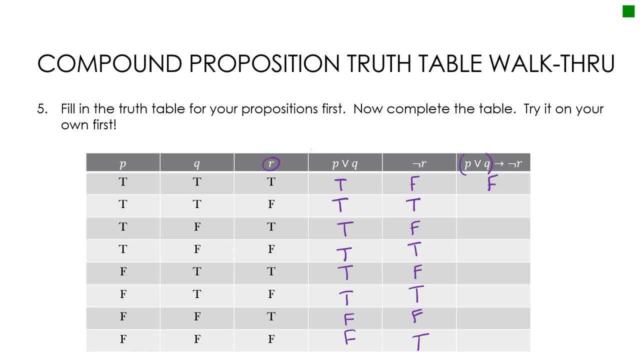 false, because not R is false. This one we have true. true, so that is a true one. This one we have true, false. that is false because if P or Q is true, then not R must be true. Again, this one must be true. This is false. this is true. We have two falses. Remember, that's that tricky one. 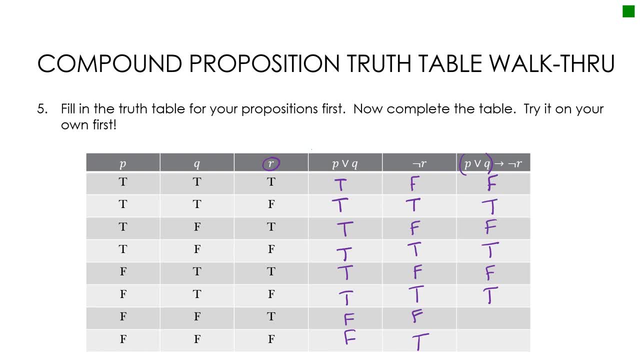 because the if part of our statement is false, then we don't care what happens here, and if the if part of our statement is false, then we don't care what happens. So that is my solution, which I have for you here on your next slide. So this is the final solution for 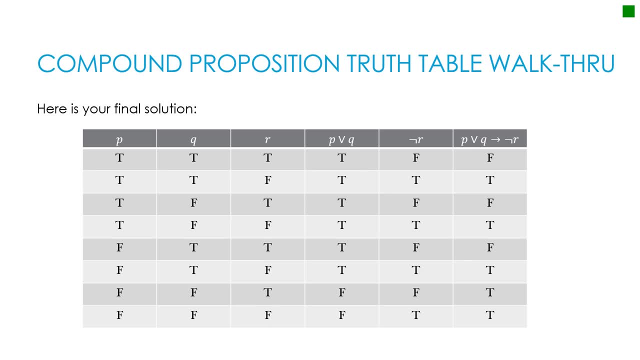 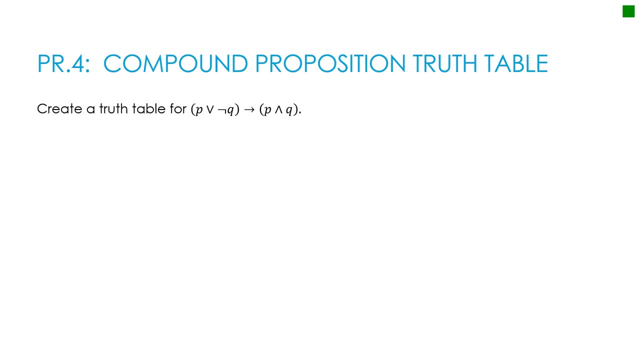 if P or Q, then not R. Of course, I wanted you to have the opportunity to try one completely on your own, and so this is that question for you. This is P or not Q? or if P or not Q, then P and Q. So obviously there. 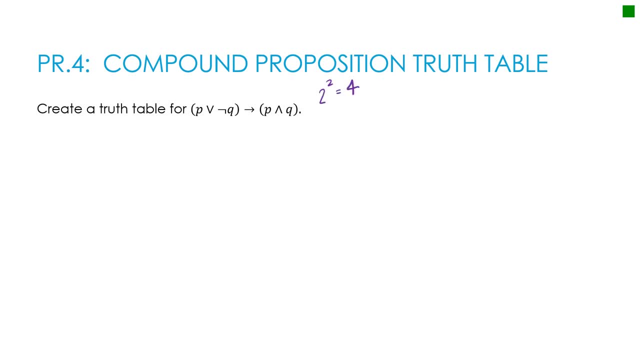 are only two propositions, which that means two squared or four rows. I will let you determine how many columns you should be using. So go ahead and do your entire truth table and then press play and see how you did. Okay, I'm going to get started. so if you did not, press pause and try it on your own. 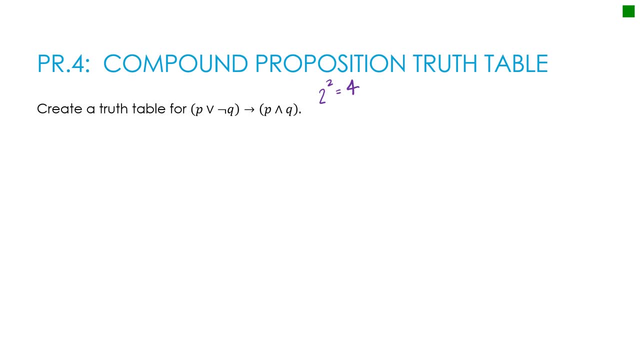 well, shame on you. All right, so we know we're just going to have our four different rows because we only have our four different truth combinations. for our two propositional statements, P, Q- Then I need a column for not Q because, as I said, if P or Q is true, then not R must be true. So this is: 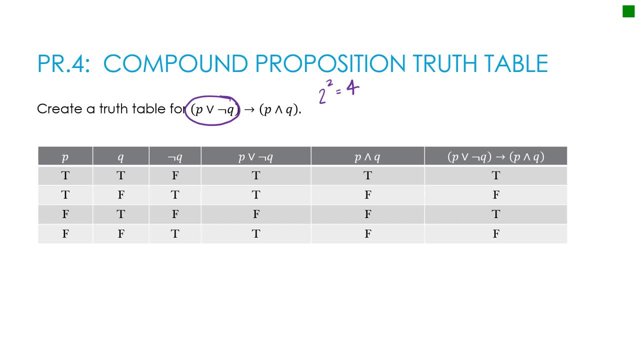 because as I'm looking at this first combination- here I'm looking at P or not Q- then I need to know what not Q is. So I've now made a not Q column, and then here I'm looking at P or not Q, And so 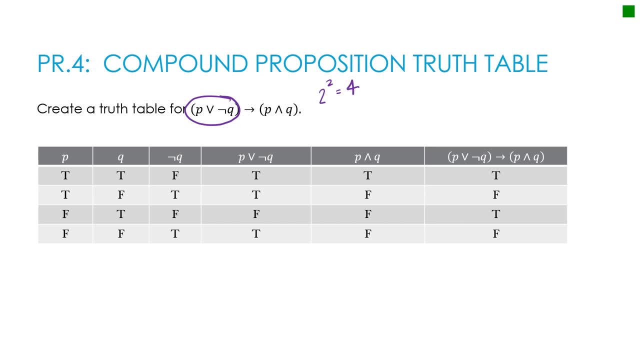 true and false gives me true. true and false gives me true, false and false gives me false because, remember, I just need either one of them to be true. and then false and true gives me true because one of the two is true. 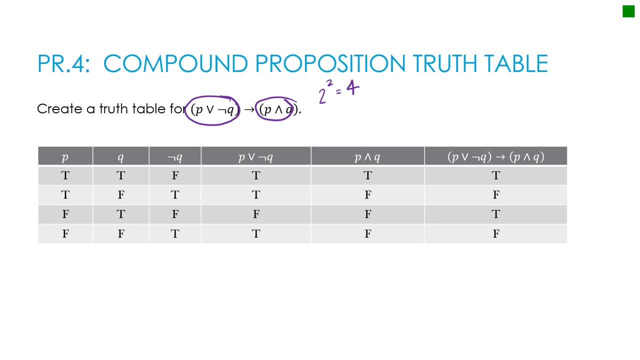 All right. so now we have that one. I'm looking at the solution to this one: P and Q. Remember, for P and Q, I need them both to be true, and the only place they're both true is right here All. 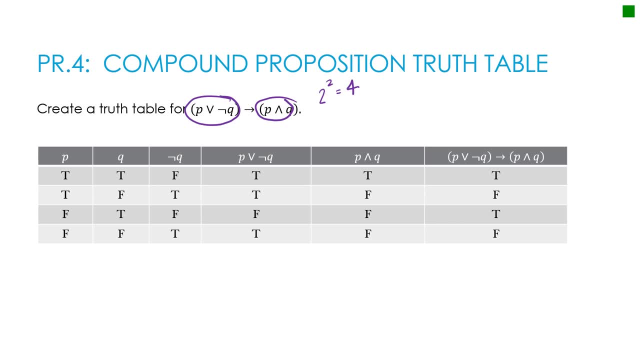 of the rest of them are false. So that, hopefully, was a very easy column for you to figure out. From here I'm looking at: if this, then this, So that is what I'm determining for my final column, And so I'm saying: 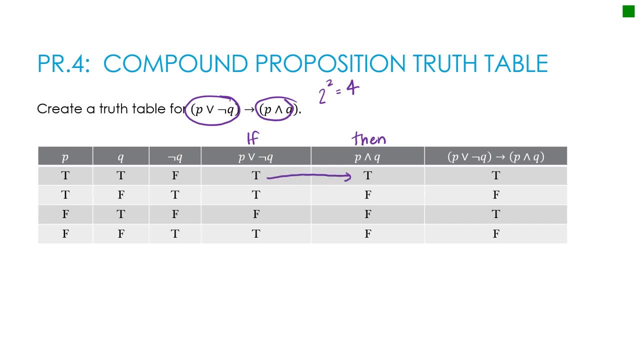 if this is true, then this one should be true. So if P or not Q is true, then P and Q must be true. And that's what I get here: true, true, This one. I start with true, but I end with false, and that's no good. So notice, my answer is false Here. I begin with.